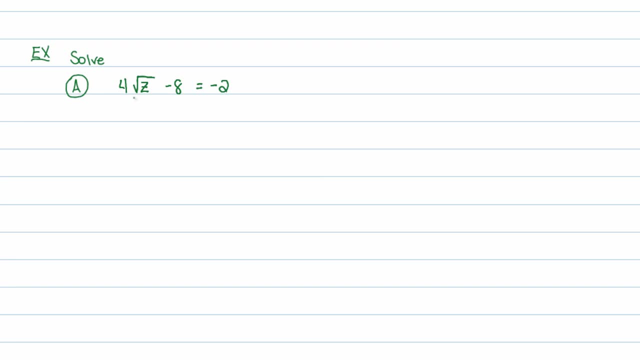 I just see if there are more than one, if more than one term contains a variable. but nope, only one term contains a variable. So that means I'm going to untie this knot. Let's list out what happened to z. The first thing that they did to kind of throw us off the 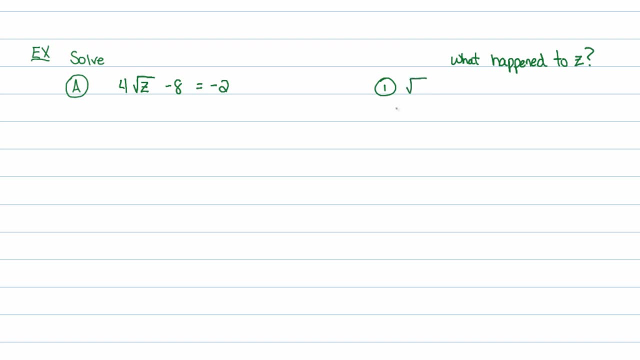 trail of finding what z is. they took the square root of it. After they did that, they multiplied it by four. After they did that, they subtracted eight. Notice the order of operations that you see right here: Exponents, multiplication, subtraction. Now, that's how. 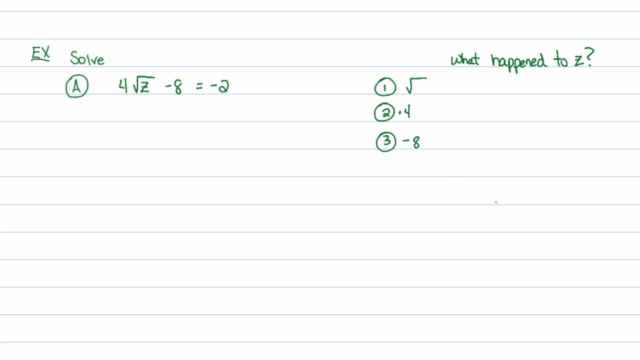 they tied this all up in a knot. To untie a knot, we just do the opposite of each of these actions, in reverse order. So we're going to do the opposite of subtracting eight, We're going to divide by four And, finally, we're going to do the opposite of taking the square. 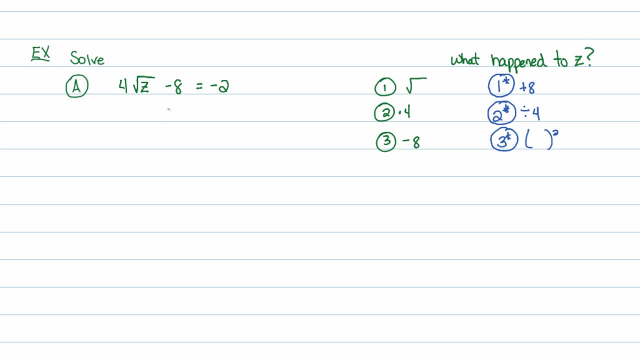 root, We're going to square both sides, So let's go ahead and do that. Add eight to both sides And we get this wonderful four times. the square root of z is equal to six, And now we divide both sides by four. Just following my little list of things to do here. Four: 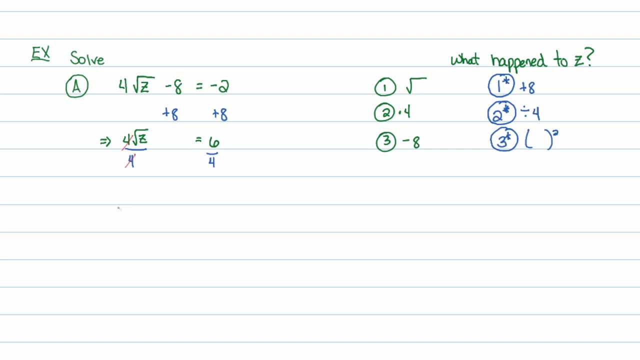 over four just becomes one, One on the left hand side by design. So we get the square root of z on the left hand side. On the right hand side this fraction will reduce. That's three halves. And finally I tell myself I'm going to want to square both sides, I'm going to go ahead and do that. 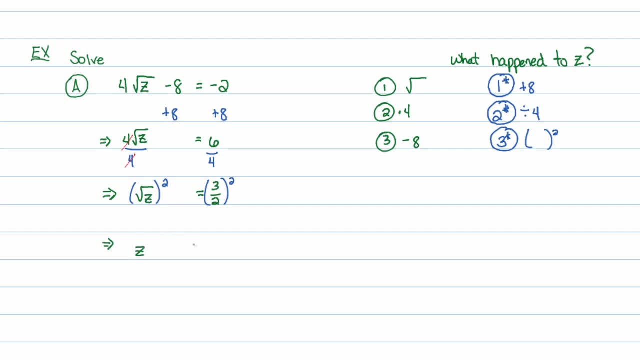 So in the end I get that z is equal to nine fourths. Now, always what you should do is check your answer. When you end up squaring both sides of an equation, you must check your answers. So please do that here. It'll be a very quick check. Just find out what. 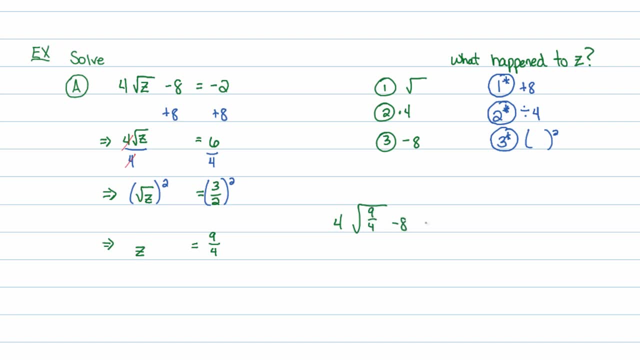 four times the square root of nine fourths minus eight turns into: Well, that's four times. the square root of nine fourths is three halves Minus eight. Two goes into four twice. That's six minus eight, That's a negative two. That works out. There, we go Very simple. 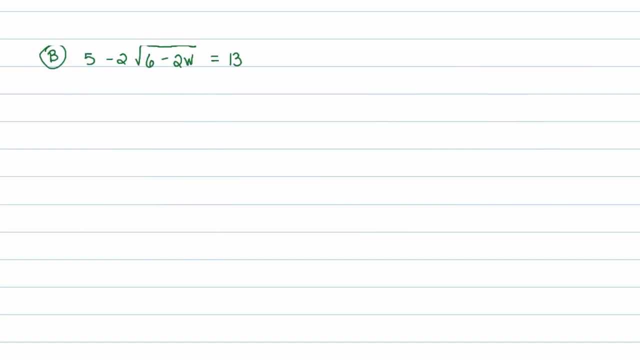 Very quick check, But you have to do it All right Again. take a look at my next victim here. Let's see Any fractions, No, Any decimals, No Great. Can I clean up the right hand side? Nope. Can I clean up the left hand side? Not. 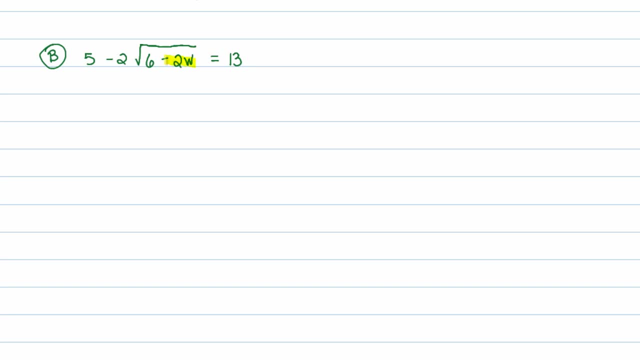 really, If you look inside this square root here, those two terms will not combine, So that's stuck. And on the outside these are not like terms. This is a five, This is two times junk, So these two terms cannot combine. That two has some issues attached to it, So 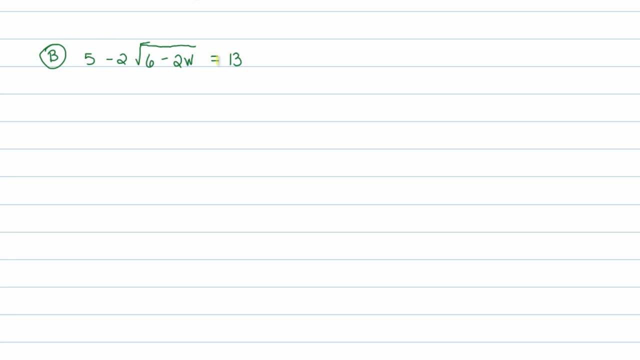 we can't combine terms. Finally, I just take a look around and see how many versions of my variable, how many occurrences of my variable there are. There's only one occurrence right there, So that means I can untie the knot. There's no special technique needed here. 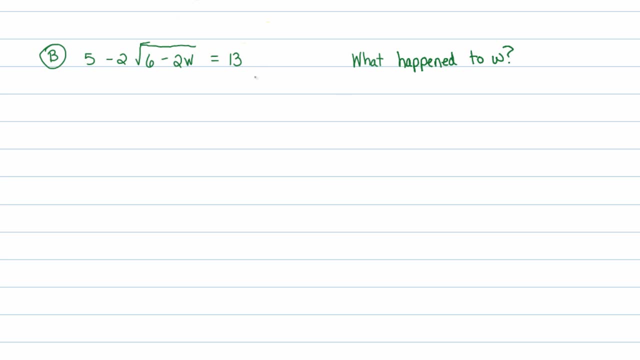 So let's list out what happened to W. As I look through this, the first thing that I see is that I have two times junk. So that means I can untie the knot. So that means it got multiplied by a negative two. So the first thing I see is it got multiplied by. 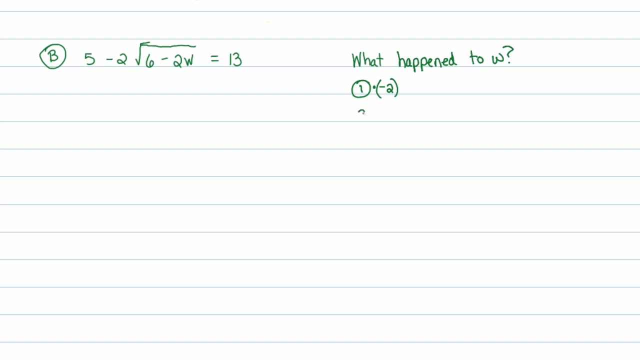 a negative two. After it got multiplied by a negative two, they added six to it, whoever they is. Then they took the square root, The reason why I know that you're thinking. wait a second, isn't this the order of operations? Should we take care of exponents first? What? 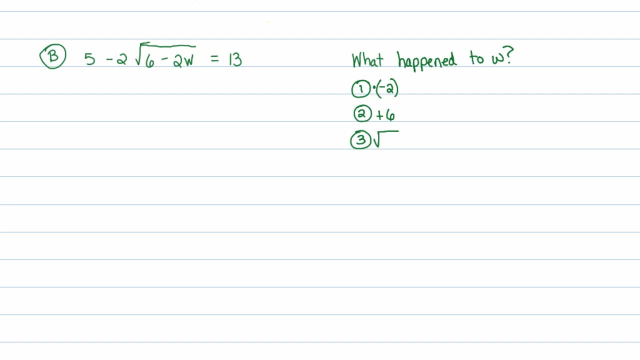 you're doing is you're centering on W. So you start with W and say: what's the first thing that happened to it? Oh, it got multiplied by that negative two. So what you're doing is you're finished. How could you go at me and push this here? It got lunatic. 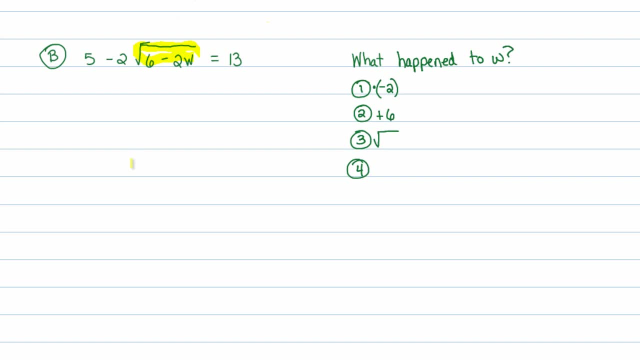 into my way. You got me a negative three. you got me a negative two. Is this working? How could you move these around? Here's how it Pavlovalov loses. You took the square root, Write that down. They multiplied it by a negative 2.. 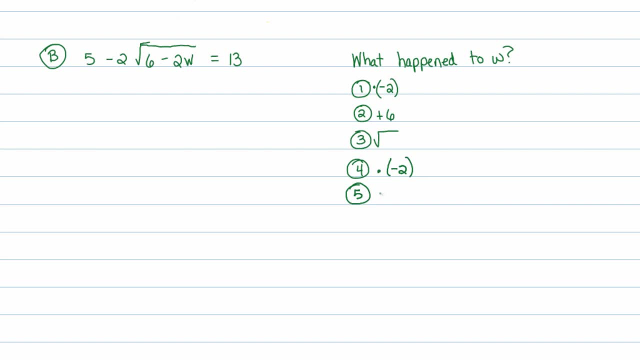 Finally, a lot of things they did. They added 5 to it. 5 out front means adding 5, plus 5.. So let's go ahead and untie the knot by undoing every single thing here, doing it in reverse order. 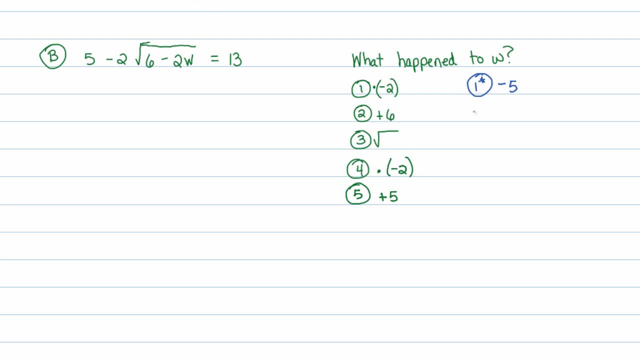 So let's see: Instead of adding 5, we'll subtract 5.. Instead of multiplying by a negative 2, we'll divide by a negative 2.. Instead of taking the square root, we'll square. Instead of adding 6, we'll subtract 6.. 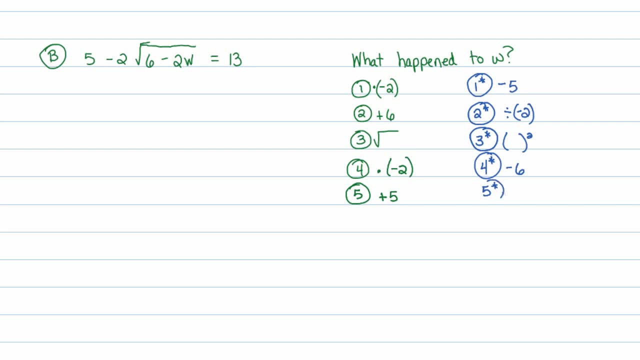 And instead of multiplying by a negative 2 again, we'll divide by a negative 2 again. Alright, let's do this. First thing I have on my list is subtract 5 from both sides. If I do that, I get this beautiful negative 2 times the square root. 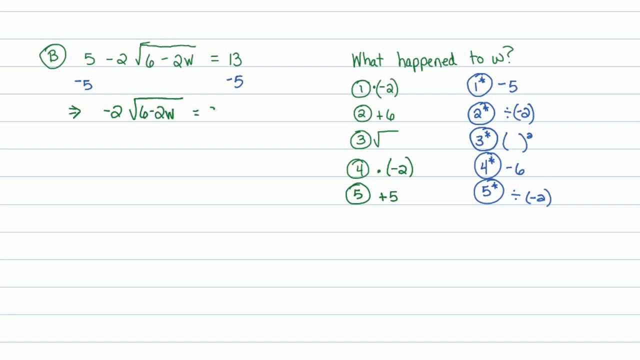 So the square root of 6 minus 2w is equal to 8.. Now there is something that should be said. Well, we'll see it in a moment. Next thing that we're going to do is divide both sides by a negative 2.. 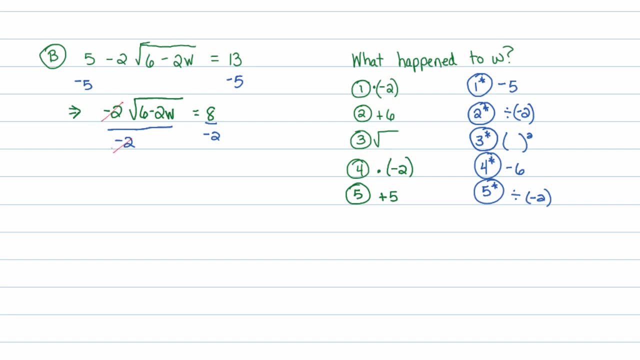 And you see on the left-hand side the negative 2 over a negative 2, that turns into a 1.. So this becomes the square root of 6 minus 2w. So the square root of 6 minus 2w is equal to a negative 4.. 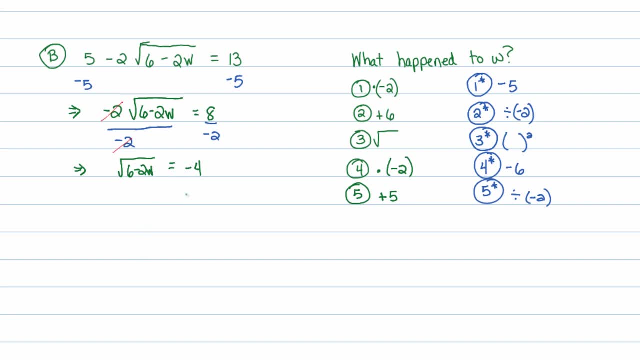 Now pause this video for a moment and see why there's no solution to this. If you don't see why there's no solution to this, then follow me forward. It's always important, or maybe not important, but always a good tactic when solving radical equations. 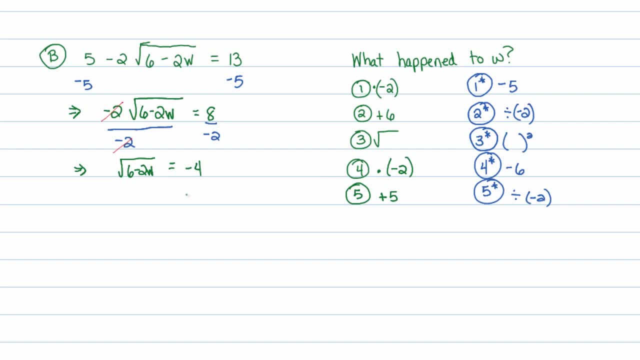 to check, once you get the square root of junk is equal to a number, To check to make sure that number is positive, because square roots can only return positive numbers. I already know right now: there's no solution. There's no solution to this. 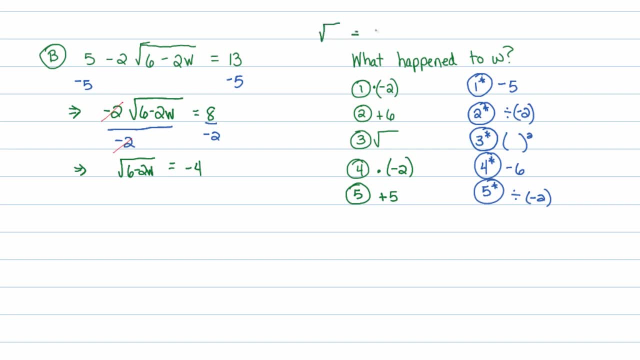 Because a square root always equals- well, basically, is always greater than or equal to 0. A square root of stuff is always greater than or equal to 0. But here we have: the square root equals to a negative number. Can't happen, so there's no solution. 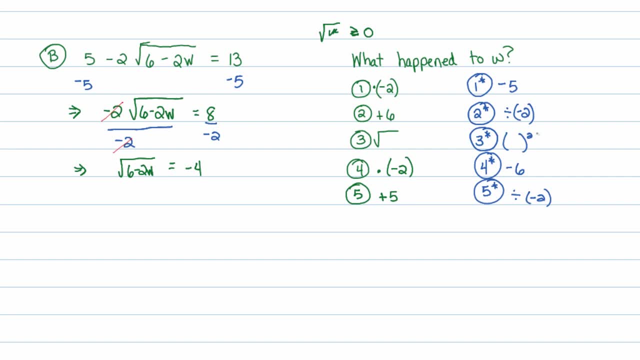 But let's suppose you didn't see that. Let's suppose you didn't see that If you continue following this list of steps, we'll square both sides And you get 6 minus 2w, because the square undoes the square root is equal to 16.. 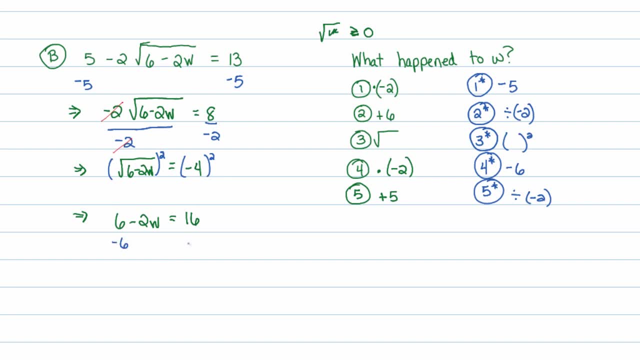 We will now subtract 6 from both sides And we'll get negative 2w is equal to 10.. And finally, we'll divide both sides by negative 2.. Sorry for the voice cracking, I am sick. So negative 2 over negative 2, that's just 1.. 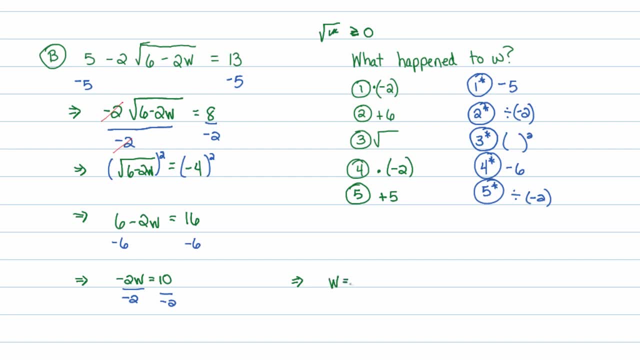 And so we get: 1w is equal to a negative 5.. Now remember what you should do. Whenever you square both sides of an equation, you have a risk of introducing an incorrect solution. So let's check the solution. So I go back to the original equation. 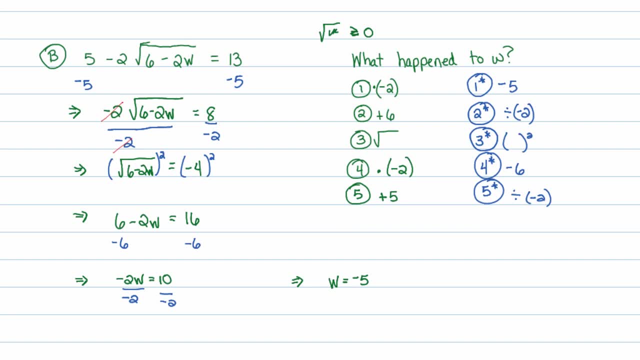 I go back to the original equation. Instead of w here, I'll go ahead and plug in to its place a negative 5 and see what happens. So if I do that, I will have 5 minus 2 times the square root of that's 6 plus 10 or 16,. 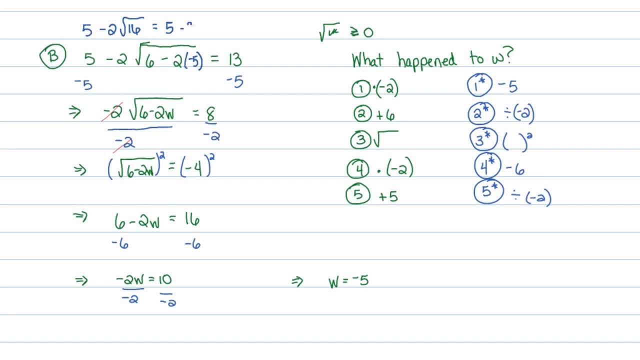 which is equal to 5 minus 2 times 4,, which is 8,, which gives me negative 3. Which is not actually equal to 13.. So that's the issue There is. this is not a solution. We call that an extraneous solution, as I mentioned in the previous lecture. 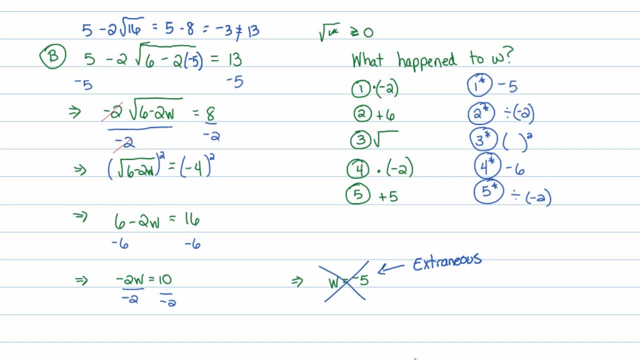 Extraneous, meaning that we've introduced it incorrectly when we squared both sides. That's why you should always check your work, But we could have noticed by the way that we were going to have no solution again way back in the beginning here. 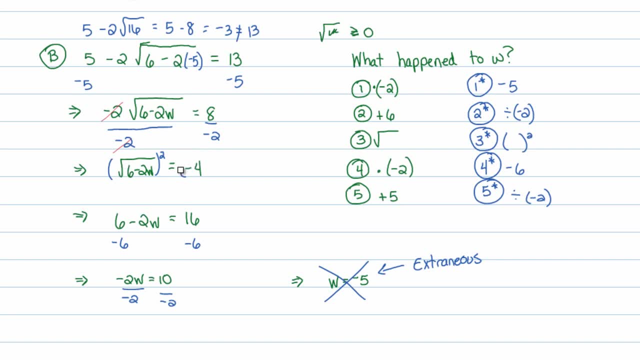 I have to change my eraser size to a very small eraser. Way back in the beginning we could have noticed that we wouldn't not beginning beginning. but at this point, right here, we could have noticed this wasn't going to happen, right. 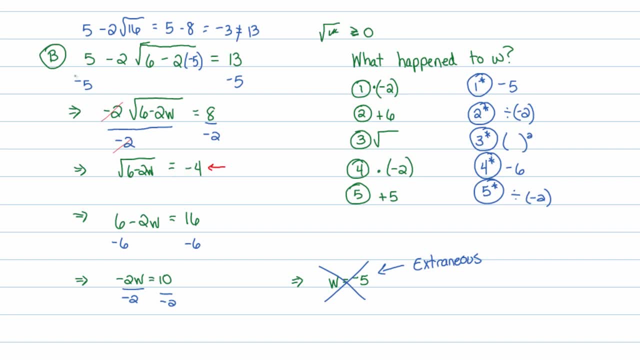 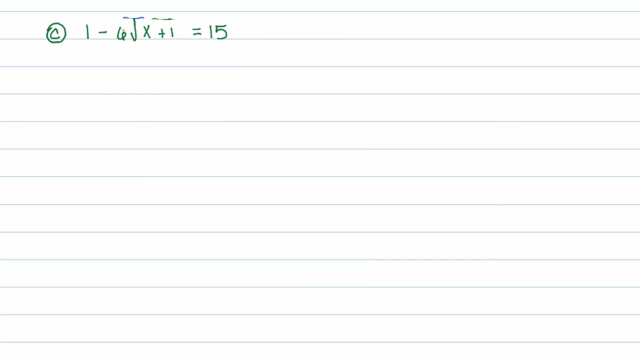 Square root of a number is never negative. So let's try another example here. In this example again, I have one version of my variable, which means that I can undo what's happening on that side of the equation. First thing I try to do is I look at both sides, see if there are fractions or decimals. 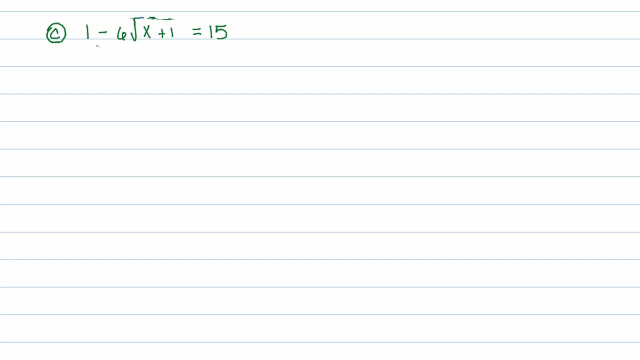 which there aren't, And then I look to see if there's any terms that can be combined. This one and this six cannot be combined because that six is tied up in a multiplication. Remember, before any type of addition or subtraction, you have to take care of multiplication. 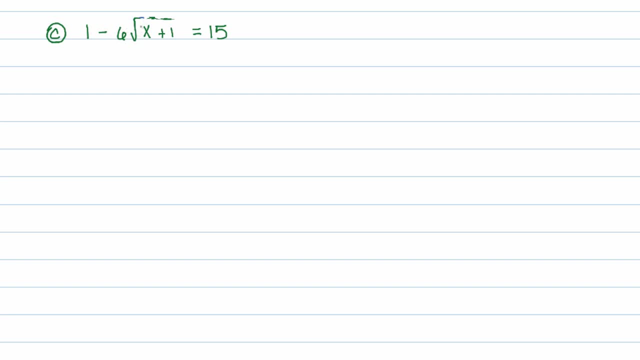 So there's no way that six times root x plus one can be simplified any further. so these two are unlike terms. So now I have to think about what happened to x. You look through this, Focus in on x first, The first thing that happened that somebody tried to do to kind of hide the value of x. 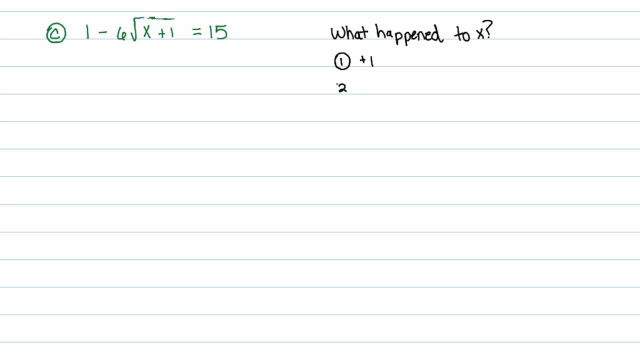 from us is they added one. The next thing they did, after they added one to x, they took the square root, And after they took the square root, they then multiplied by a negative six, And after multiplying by a negative six, they added one. 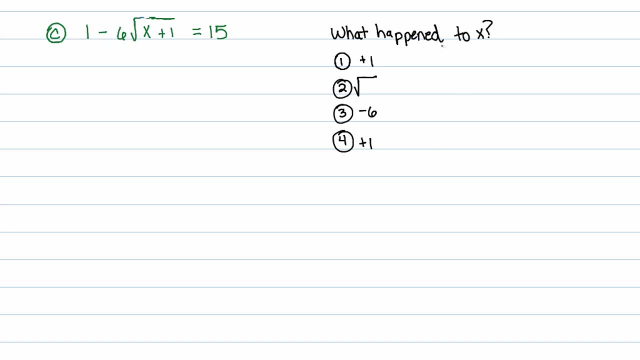 That's this last little bit right here. So again, we're going to undo this stuff in the opposite order. So I'll start up here And I have to undo the first one. I'm going to do the last thing that they did. 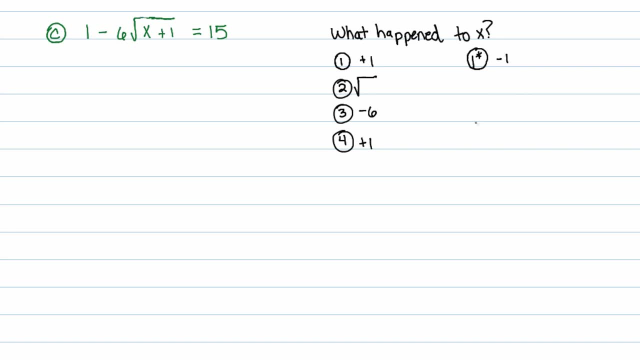 They added one here, so I'm going to subtract one from both sides. The next thing I have to untie is the subtraction of six, so I'm going to add six, all inverse operations. The next thing I'm going to do is undo the square root, which means I'm going to square. 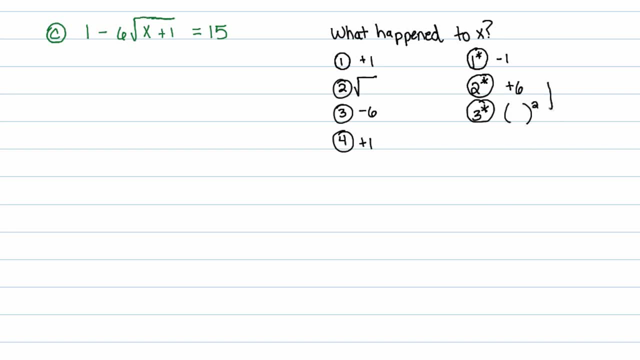 both sides. And that is the step where, in the last example we saw, we can introduce an extraneous solution. So this is cause for checking solutions always. And then the fourth and final step. they added one. I will subtract one. 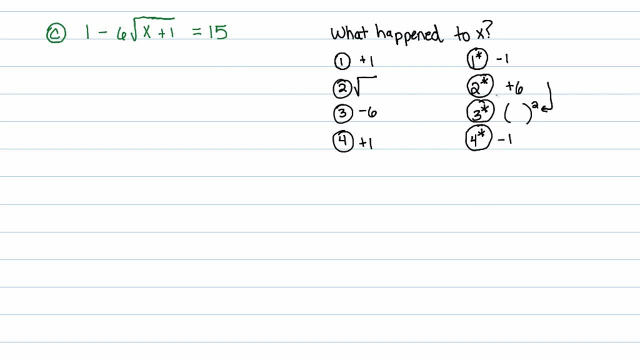 So let's go ahead and do this First step. I tell myself to subtract one from both sides. So when you do that you get this wonderful negative six square root of x plus one is equal to fourteen. And then I tell myself next thing: so this one's done. 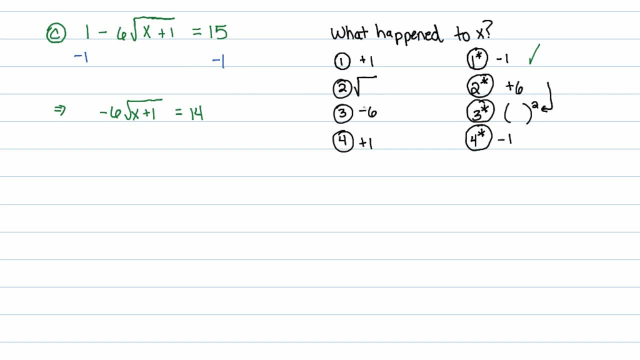 Add six, Not add six. Man, I'm probably thinking that I don't know what I'm doing here. We multiplied. I even said it. I remember saying we multiplied by a negative six in this step. So going back here, remember first thing that happened to x: we added one, then we took. 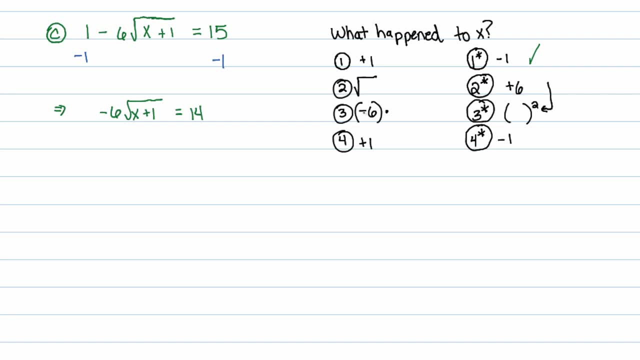 the square root. Then we multiplied by a negative six. It looked like I was saying subtraction by a negative six, so that's why I convinced myself that over here was right. Let me just erase this and put in the proper thing here. So let's see. 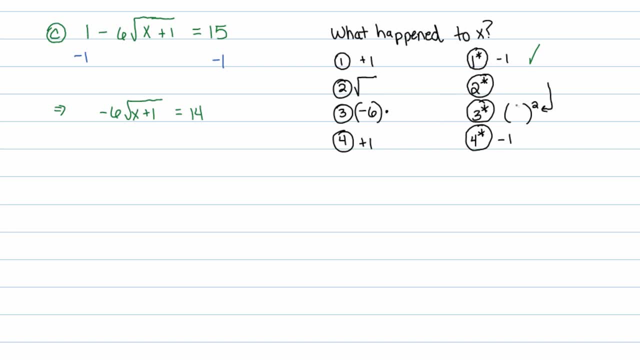 We would undo addition, We would undo multiplication by dividing both sides. There we go. Yikes, That was near tragic. So I'm going to divide both sides by a negative six And you see, the negatives will cancel. Six over six is just one. 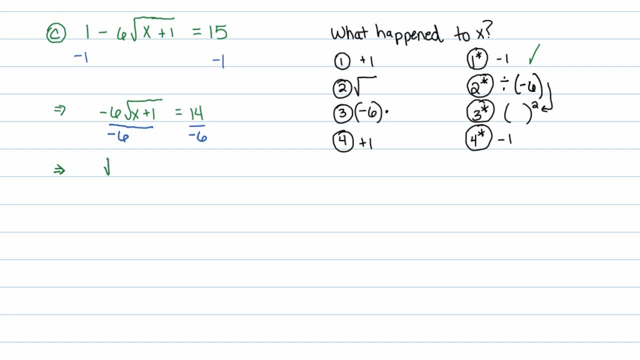 So the left hand side turns into the square root of x plus one, The right hand side. I'm going to reduce that fraction. Both top and bottom are divisible by two, So that will be a negative six. So I'm going to do that. 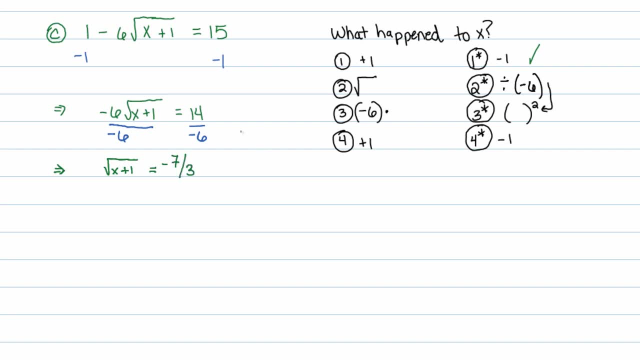 Seven thirds. And remember it's always just good form to write negatives in numerators or out front. A lot of people do not like negatives in denominators, So it's just good form to leave it out front, Not that it is incorrect. 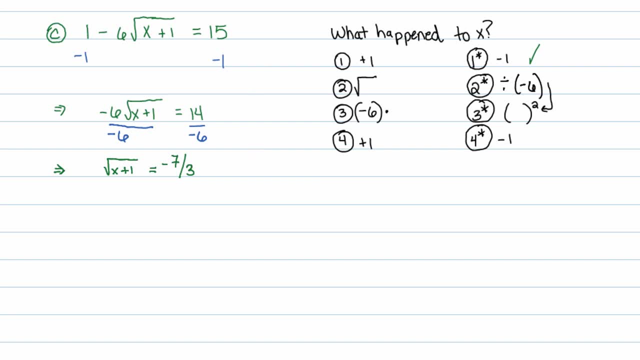 It's just good form. Now, before I go any further, I just want you to again: once you get to a point where you have a square root of something with a variable equals a number, you should always check to see if that's feasible. 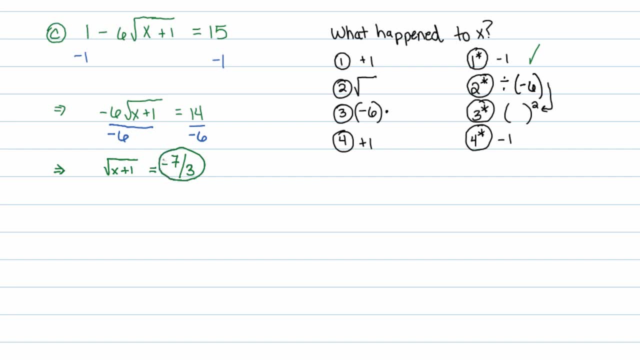 Notice that this number here is negative. Square roots never equal negative numbers, equal negative numbers or negative real numbers. i should say so. therefore, there will be no solution. i already know right now there's going to be no solution. however, i do have a lot of students. 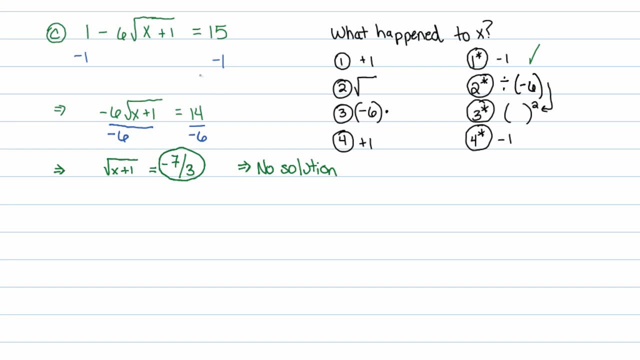 that just continue forward blindly, and which is understandable. you just kind of- especially during an exam, you don't really think. you're just kind of moving along. so if that's the case, let's see what would have happened. well, let's see. i tell we're done with this step. so the next step was: 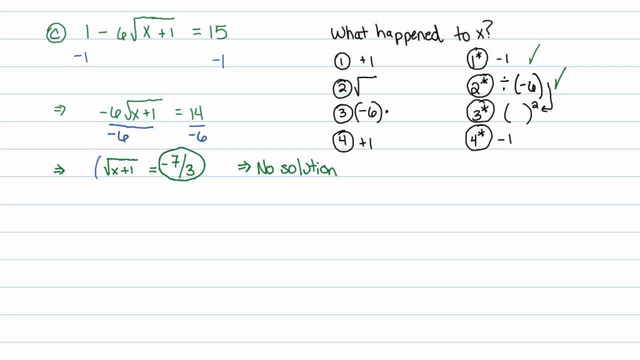 to square both sides. so if we squared both sides we would get on the left hand side the square and the square root cancel. we get x plus one on the right hand side negative. seven squared is 49, three squared is nine, and then subtract one from both sides. so let me check this off and i'll. 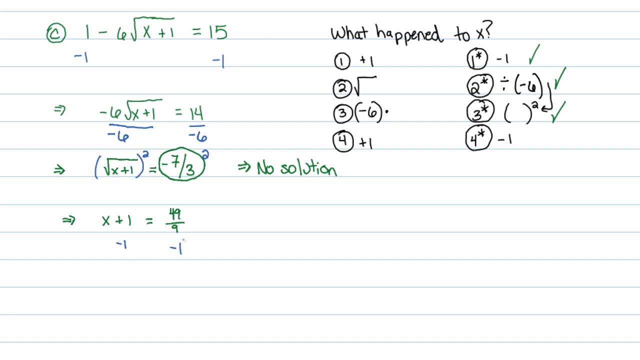 subtract one from both sides. subtract one, subtract one, now one is the same thing as saying nine ninths. so i'm subtracting nine ninths from both sides. so this gives me that x is equal to 49 ninths minus nine of those ninths. leave me with 40 of those ninths. but remember, always check your work, because 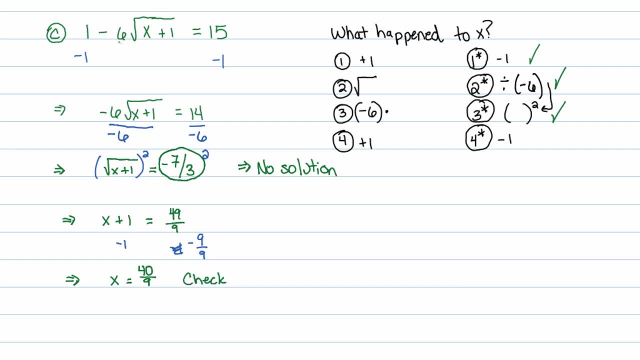 you squared both sides. so if you try to check this work, it will not actually work out, because what happens is you get one minus six times the square root of 40 over nine plus one, which is the same thing as one minus six times the square root of 40 over nine plus one, which is the same thing. 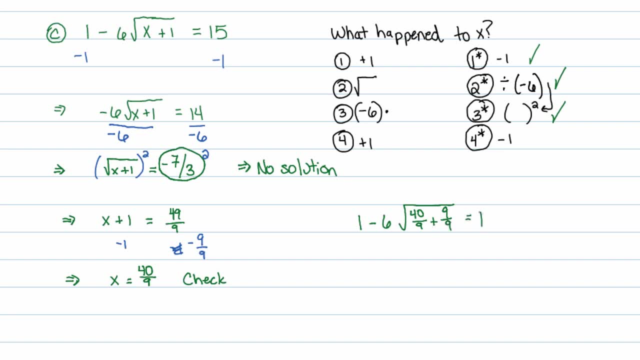 is nine over nine. well, let's go ahead and simplify this down. that's one minus six times the square root of 49 ninths, and square root of 49 ninths is seven thirds, six times seven thirds. well, three goes into six twice, so that's going to be 1 minus 14, which is going to be a negative 13, which is not. 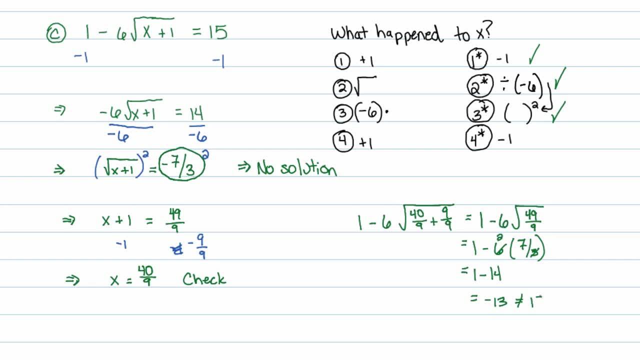 equal to 15, so that's an extraneous solution. again, no solution, right. but you know how much? did you notice how much extra work we had to go through to solve this when we didn't take the time to recognize that a square root can't equal a? 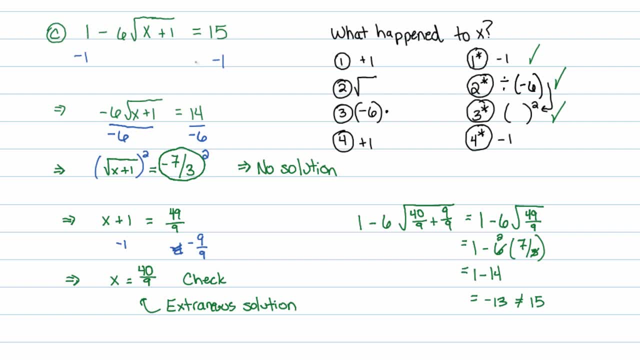 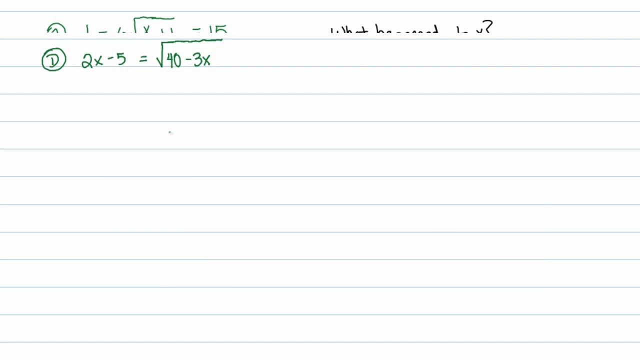 negative number. so whenever you're solving radical equations, always good to keep out. keep an eye out for that. now we have our first foray into a radical equation that has two different versions of our variable. what i mean by this. well, i'll just show you now. 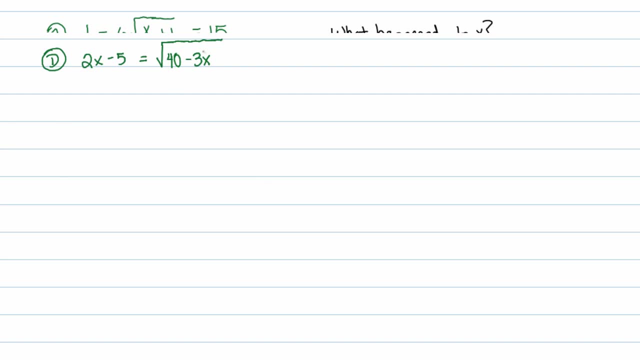 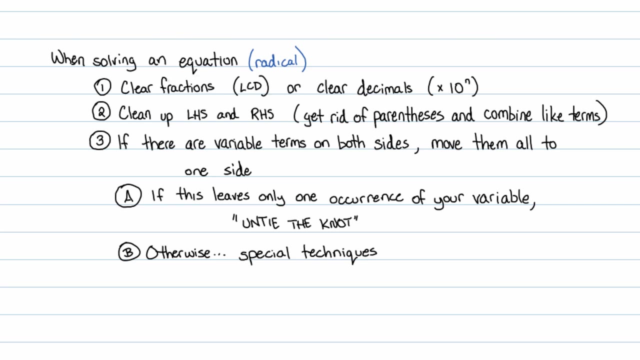 recall that we had mentioned a list of techniques, or maybe i shouldn't say list of techniques, but a list of ideas when you want to solve an equation, clear fractions or decimals, clean up left and right hand sides by getting rid of parentheses and compiling like terms, if you can, and then if. 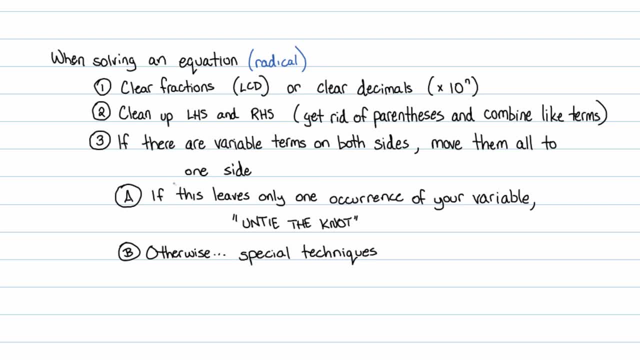 there are variable terms on both sides, move them all to one side once you do this. if this leaves you with only one occurrence of your variable, untie the knot. otherwise you have to resort to special techniques and with radical equations, the special techniques you're gonna use is to isolate one of the radicals. 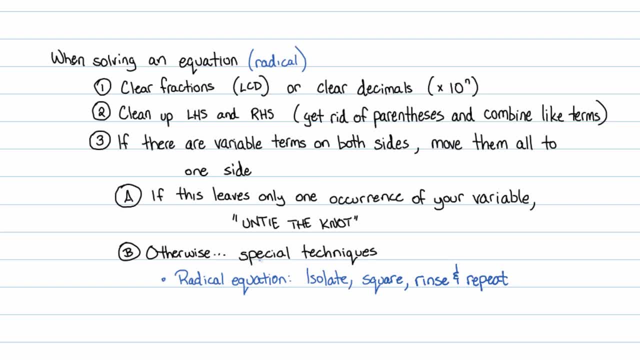 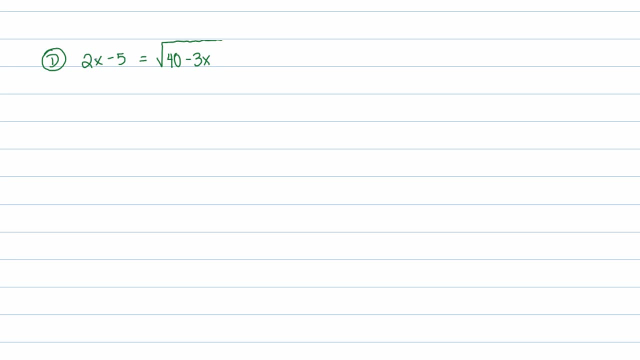 square, both sides, rinse and repeat, meaning you'll end up with another radical, isolate that and also square again. this process might continue another two times, or something like that. so, looking at this example, there are no fractions, no decimals, and on the left hand side I cannot combine like terms. There are no like terms On the right hand. 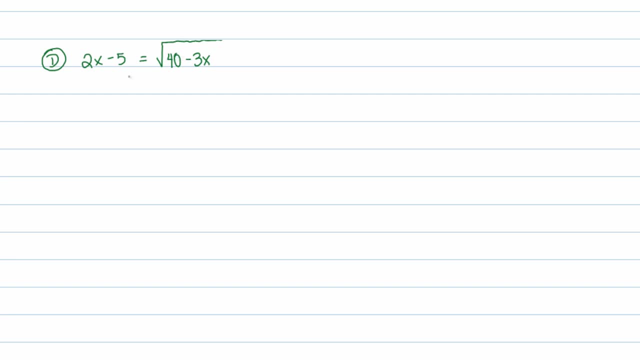 side. there are no like terms, And I also see that if I were to try to move anything between sides, nothing would combine. In other words, as an aside, if I subtract 2x from both sides, I'd get this Some picture with a root 40 minus 3x on the inside of it, and then I'm 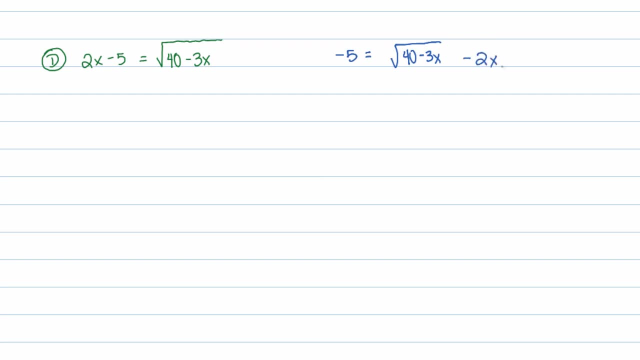 subtracting 2x from that And these two terms can't combine because this 2x is free outside a radical And this 3x here is inside a radical, so they cannot be combined. There's no combining, These are not like terms. So once I realize that, no matter how I kind of move things here. 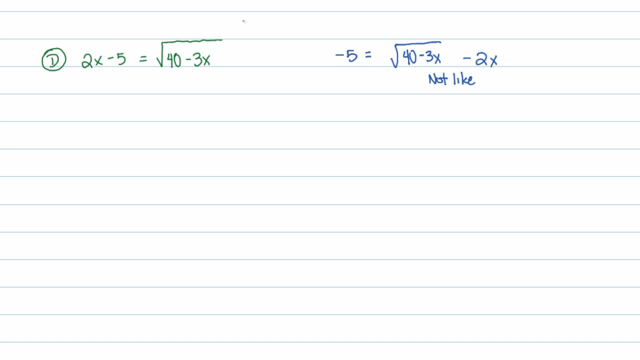 I cannot get these terms combined. I immediately think: isolate a radical, square both sides, and I might have to do something. I might have to do something. I might have to do something. I might have to isolate a radical again and square both sides again. It might have that. 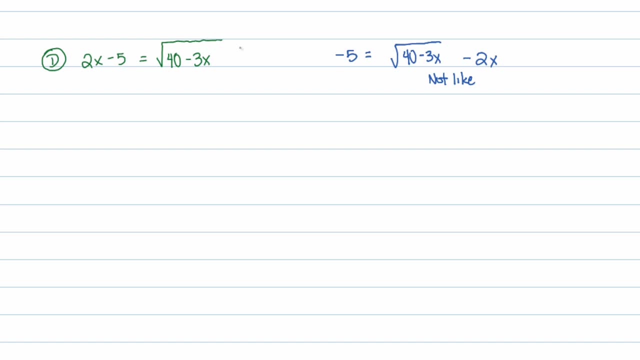 process might continue. If I'm lucky, I won't have to do that. So in this case you cannot use our untie the knot technique yet. It may turn out that you can later on, but at least at this point, because we have two different versions of our variable that will not combine. 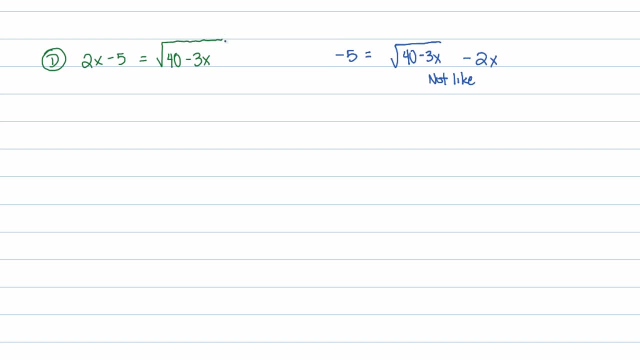 you cannot use that untie the knot technique, So I'll start by squaring both sides, because that's the only way I'm going to get rid of the radical. Now remember: 2x minus 5, quantity squared, is the same thing as 2x minus 5 times 2x minus. 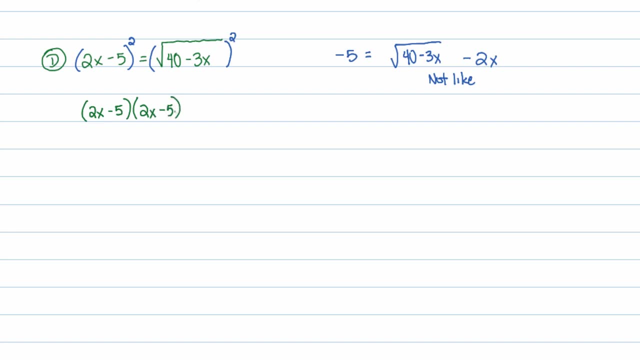 5. Be very careful of that, because I for one, as an instructor, hate when students write that as 4x squared plus 25 or minus 25, and I mark off all credit when students do that because these are basic algebra skills. You should know that this means an object times. 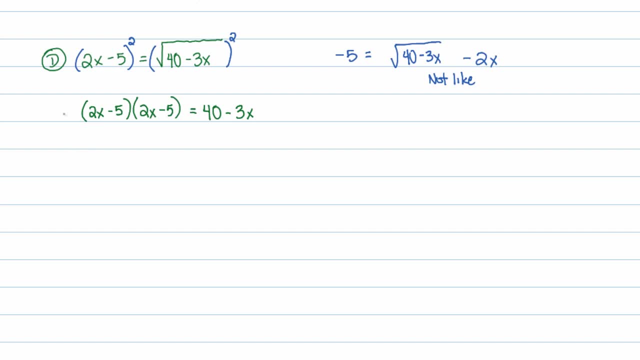 itself. I'm going to do it very quickly. Distributing through, we'll get 4x squared minus 10x, minus another 10x, so that's minus 20x plus 25 is equal to 40 minus 3x. Again, I'm going to move. 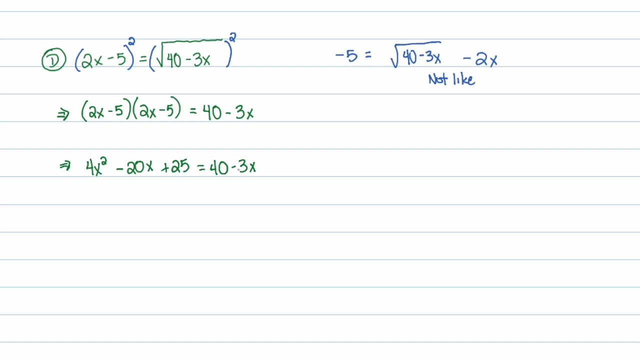 all variable terms to one side. So I'm going to add 3x to both sides. I'll even write that in here: Add 3x to both sides. Notice how I stack it. So I look at the variable terms that have only a single power on X. So this gives me. 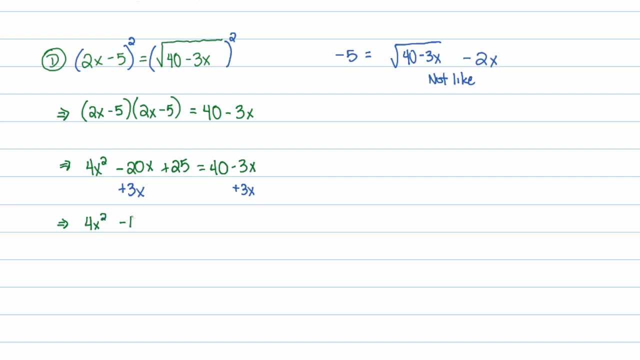 4x squared minus 17x plus 25 is equal to 40. I take the time to look through this and see if anything else on the left hand side will combine or anything else on the right hand side will combine. That's a big no so far. 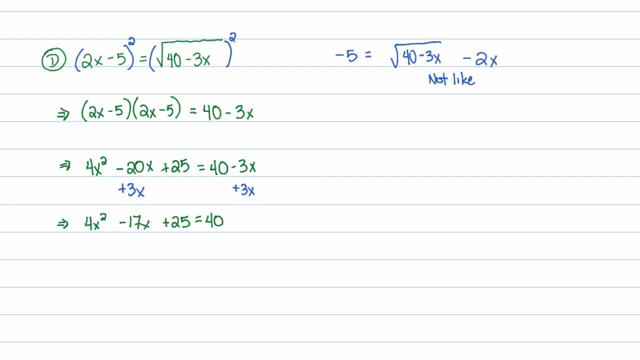 Then I ask myself: how many different versions of my variable do I have here? Well, I have two. All right, You can see, I have 15.. different versions: i have an x squared version right here and a single powered version of x right there. that means i still have. this is still a special technique to solve this. 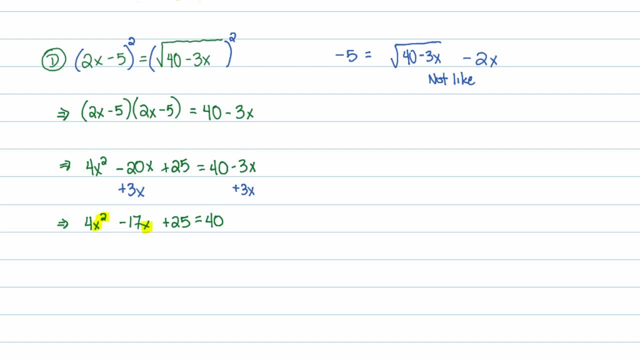 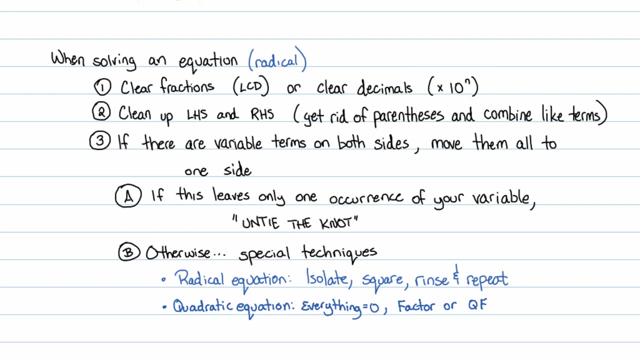 equation. in other words, i can't say what happened to x and list out all the the things that happen to x. i have to resort to special techniques, and this is quadratic and the special techniques for quadratic equations. we're first going to isolate everything on one side, so move. 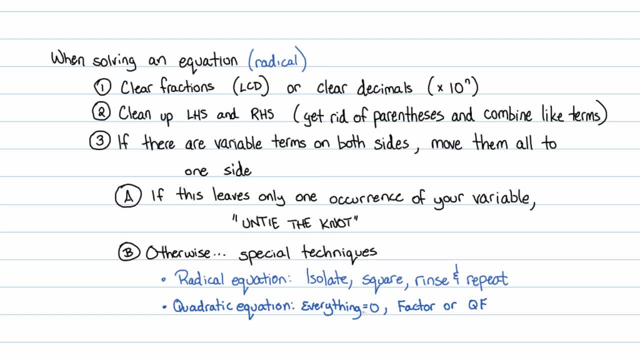 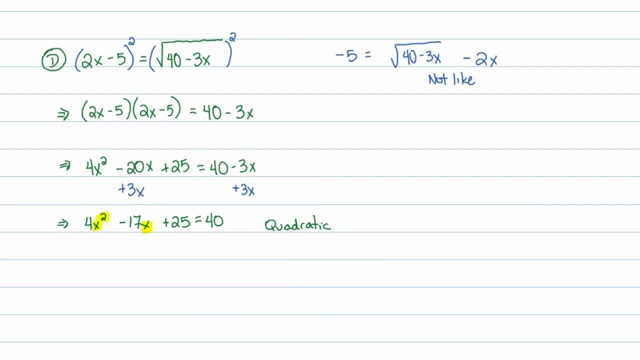 everything over to one side and set the right hand side, of the left hand side, whichever you prefer, to zero and than you're going to either factor that quadratic which can be factored or use a quadratic formula. so lets go ahead and move this forty over subtract. 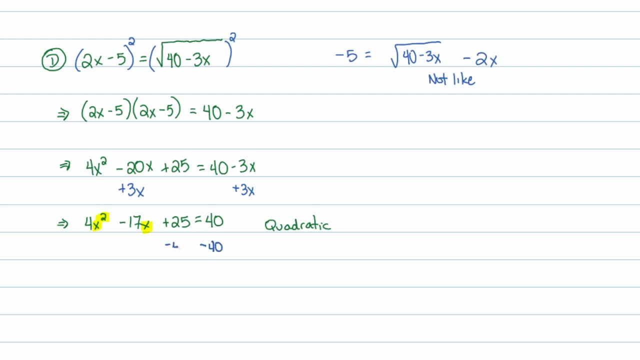 forty from both sides and i get, lets see. this implies that i have four x squared minus seventeen x, see 25 minus 40 should be a negative 15, I think zero. now I'm going to see if that factors. I know that four factors into two and two, or four and one and 15. 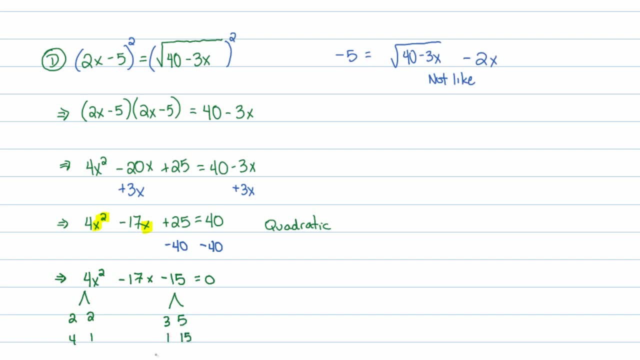 factors into three and five or one in 15, so not very many choices. that means that this should be a quick factorization. if it does factor, let's try the two and two first. so two and two and we'll see if three and five fit in there nicely, if I. 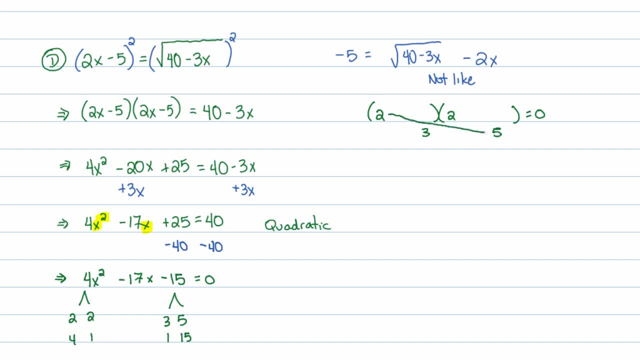 chose three and five. let's see: two times five is ten, three times two is six. no way to combine ten and six to become seventeen. so this is not the proper factorization. I'll just go ahead and cross that out. so let's try the one in. 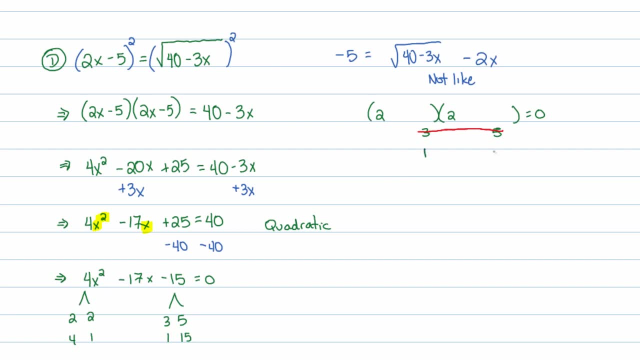 15. now, two times 15 is 30, 1 times 2 is 2. so 30 and 2. no way to combine those to become a negative 17. so again, I'll just take those two options out. so obviously the factorization, if it does factor, doesn't start with a two and a two, because I've 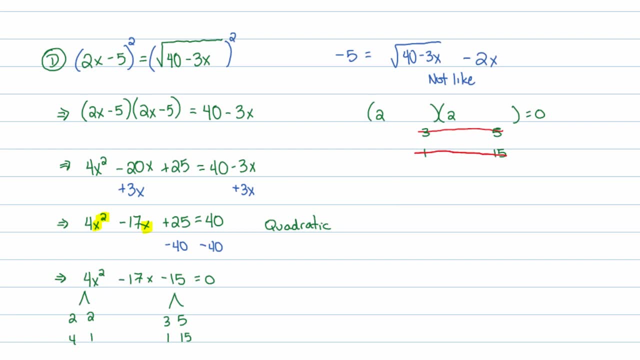 already wasted all my tries for two and two, so let's try the four and one. factorization four and one. by the way, these were supposed to have X's on them. I just kind of insert them later on. so let's try this now, because these two numbers are 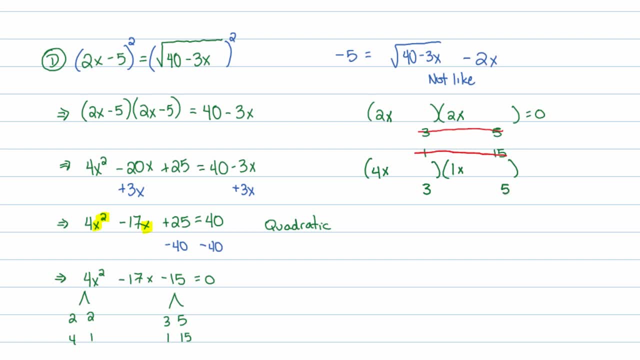 not the same. when you write three and five, you have to also write 5 and 3. it makes a difference. so let's try this: four times 5 is 20. 3 times one is three, twenty and three. is there any way to make twenty three become seventeen? yep sure. 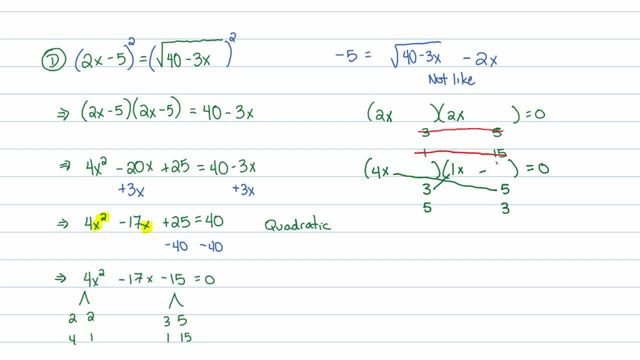 is. We want actually a negative 17,, so I'd like it to be a negative 20 and a positive 3.. Double check your work here: 4x times 1x is 4x squared. so that's this business, right here, Let's see. 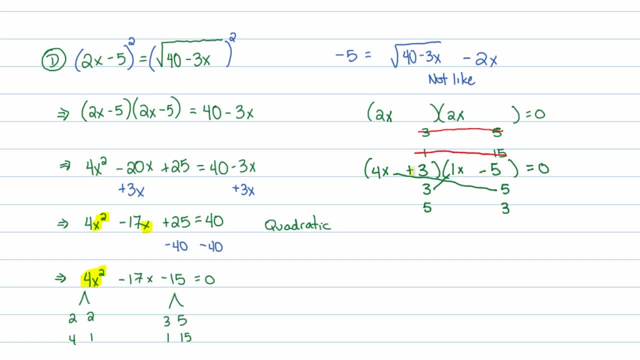 4x times a negative 5 is negative 20x, plus three more of those x's will give me a negative 17x. so that's right there. And finally, positive 3 times a negative 5 is a negative 15, that's that. 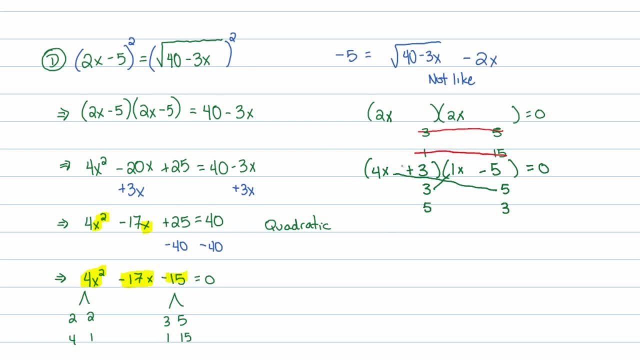 one right there. So this actually does factor to: 4x plus 3 times x minus 5 equals 0.. Now that we know it factors- and let me just erase off most of this other junk on here- now that we know it. 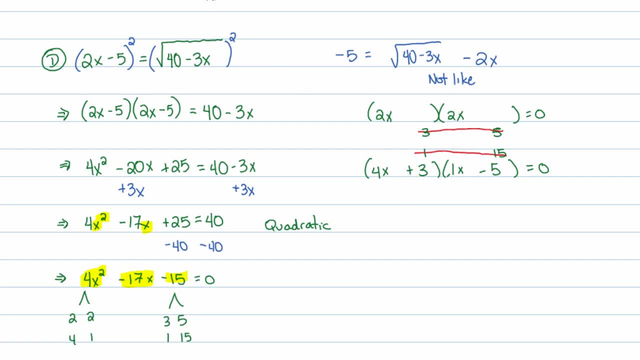 factors. we can say, using the zero factor property, that if two objects multiply to become zero, then one of them must be zero. Either 4x plus 3 is equal to 0, or x minus 5 is equal to 0. They both can be equal to 0, or maybe. 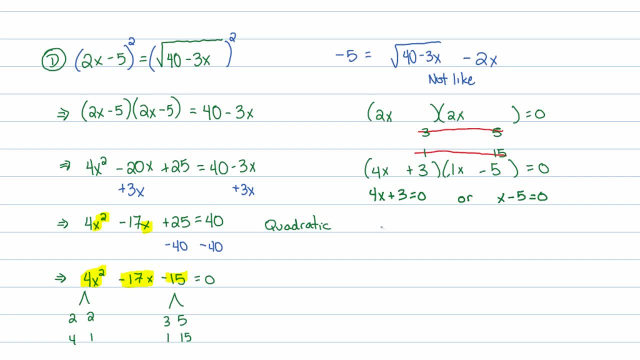 one of them is extraneous because we squared both sides initially, so we might have a wrong solution in here. Solving each of these, I'll get: x equals a negative three-fourths, or x is equal to 5. And you have to check both of those solutions in the original equation, So check. 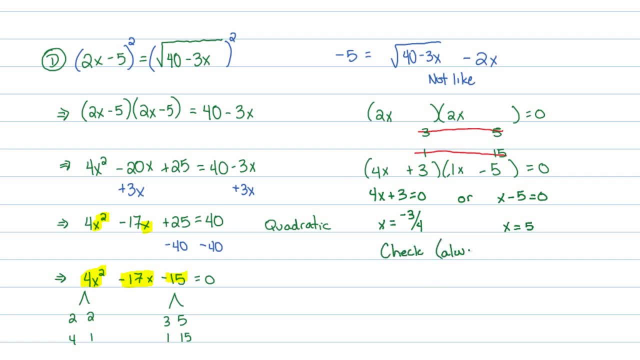 always with the original, Always in the original equation. So let me go ahead and erase off these powers here and let's take a look at this original equation. So let's do the negative three-fourths. We're just going to have to do it. So negative three-fourths if I plug that in. 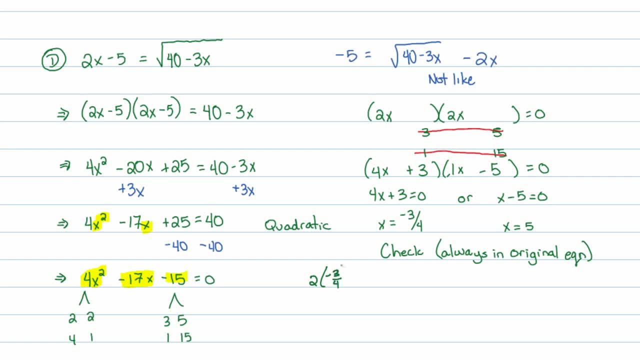 of 2 times a negative three-fourths minus 5, which, by the way, 2 goes into that 4 twice. so that's negative three-halves minus 10-halves. So negative three-halves minus 10-halves is a negative 13-halves. Now I want you to notice something here, Before I even 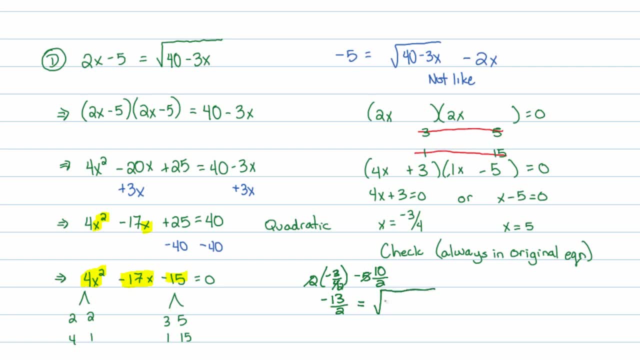 plug into the right-hand side, that's supposed to equal the square root of some number, right? I mean, when I plug negative three-fourths in there, that'll be the square root of some number. When is a square root ever equal to a negative real number? 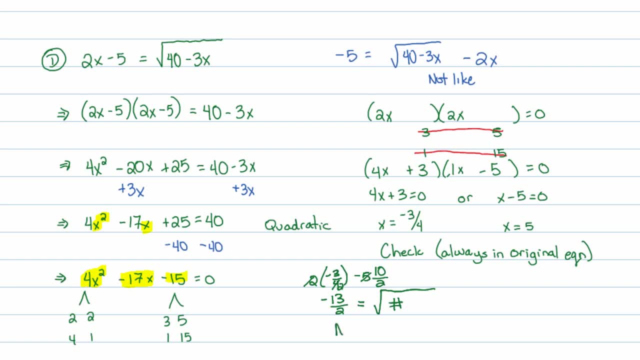 Never. So this can't be true, Not true, Not possible, I guess you could say. So turns out that we do have an extraneous solution. This one right here is extraneous. I'll cross that out. As we plugged it in, it didn't work out. You could have plugged in a number, You just would have had something. 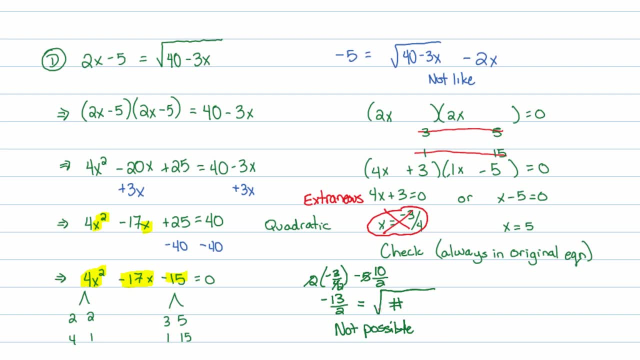 like the square root of 169 over 4,, but it still wouldn't work. Now let's plug in 5.. 5 is the easy one. So 2 times 5 is 10 minus 5 is 5.. And 40 minus 3 times 5, well, 3 times 5 is 15.. 40 minus 15 is 25.. Root 25 is 5.. Oh, 5 and 5.. Okay. 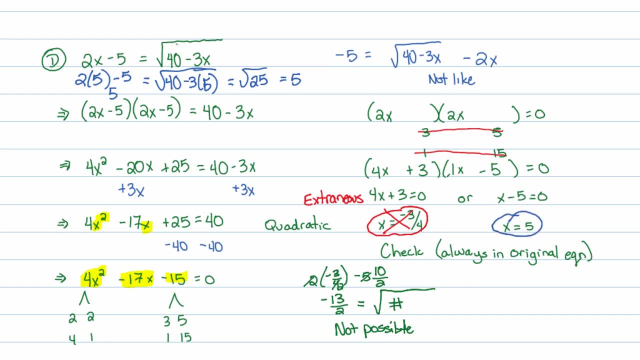 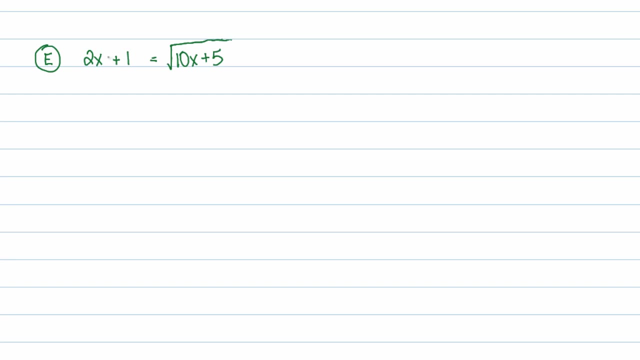 so that works out. So this right here is our solution. It's not always the case that you're going to have an extraneous solution. It just happens quite often, though, So let's try it again, Again. I already know there's no fractions, no decimals to clear. 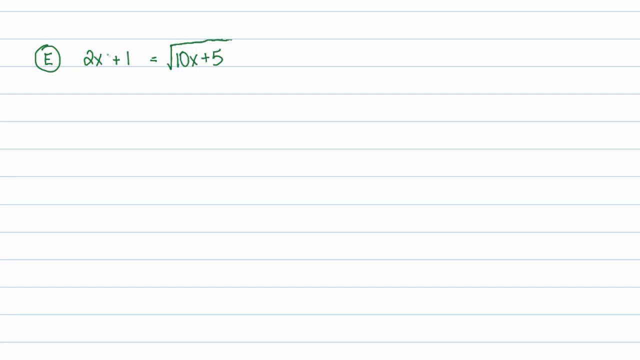 out. I can't combine like I can't. there are no like terms, so I can't combine any terms, And I know that I have to unlock this unknown from this radical. so I'm going to have to square both sides immediately And when I do that, when I square both sides, I will get 10x plus 5 on the right hand side. 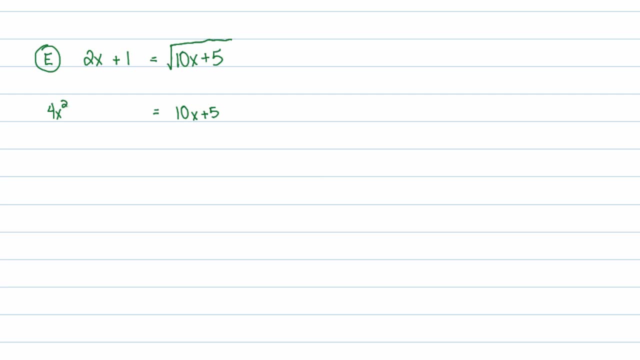 And when I square the left-hand side, I will get 4x squared plus 4x plus 1.. Notice that I didn't write it out slowly, and the reason why is because I want you, if you're confused, to try to. 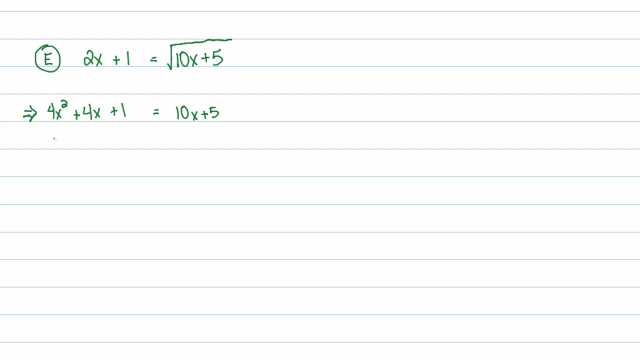 write it out yourself. I figured out how I got that. I can easily see that we're going to have two terms with different powers. on x, We'll have an x squared and an x-term. So this is going to require special techniques for solving quadratics. 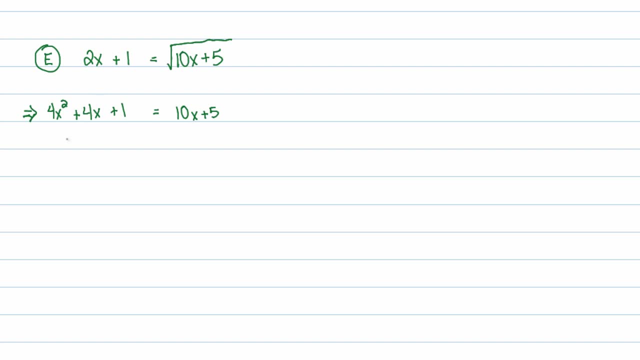 which means either factoring or quadratic formula. so let me go ahead and move everything to the left hand side. 4x squared minus 6x minus 4 is equal to 0. let me make sure my math is correct. yes, it is. i also notice right away that all these are divisible by 2, so i'll factor 2 out. 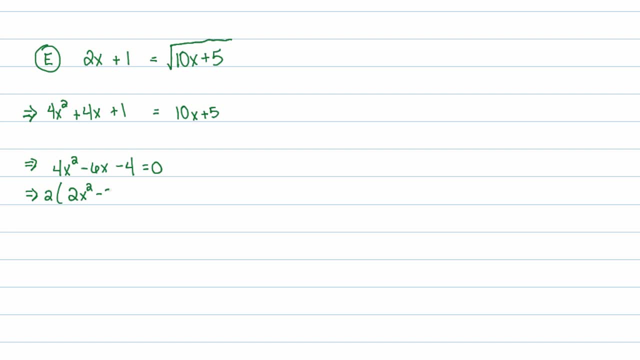 left with 2x squared minus 3x minus 2 is equal to 0, and i'll go ahead and try to factor that trinomial. i know that 2x squared is only factorable into 2x times x, so and then negative. 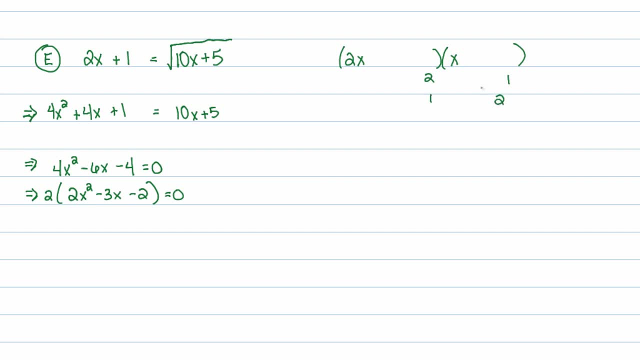 2 can either be 2 and 1 or 1 and 2. so i ask myself: 2 times 1, 2 times 1, that's 4, or, i'm sorry, 2 times 2 times 1 is 2, 2 times 1 is 2, so we have 2 and 2. any way to make that into a 3? 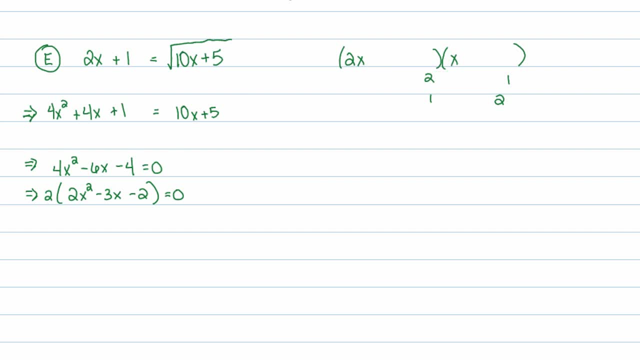 no, so that's. that's not possible. i'll cross out that one and then: 2 times 2 is 4, 1 times 1 is 1, 4 and 1. any way to make that into a 3, a negative 3? yeah, possibly. 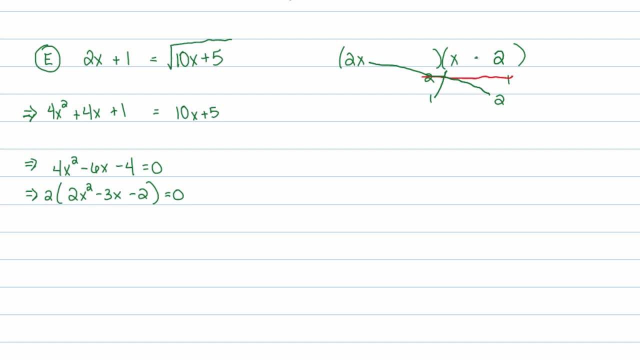 it is possible if that was a negative 2 there and that's a positive 1 there, right? because 2x times that negative 2 will give me a negative 4x plus 1x, that's a negative 3x. so this does work. 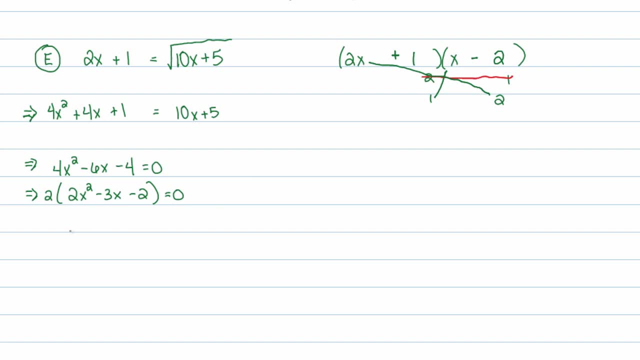 out. so when we factor this, it'll turn into 2 times the quantity 2x plus 1 times the quantity x minus 2 is equal to 0. i have 3 objects. multiplying to become 0 means either the first object is 0, which well come on 2. 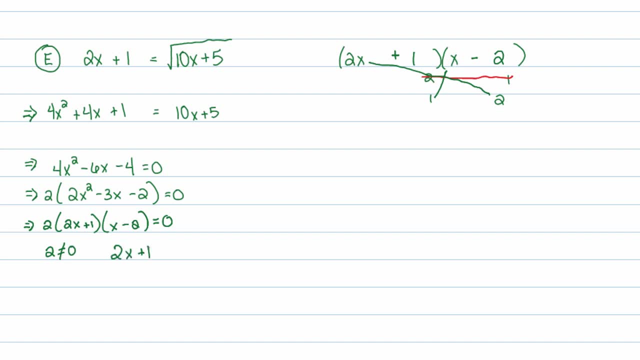 is never 0, or the second object is 0, or the third object is 0. solving for x, you get x equals a negative 1 half, or x equals 2. and remember, check by substituting these back into the original equation. so let's try. 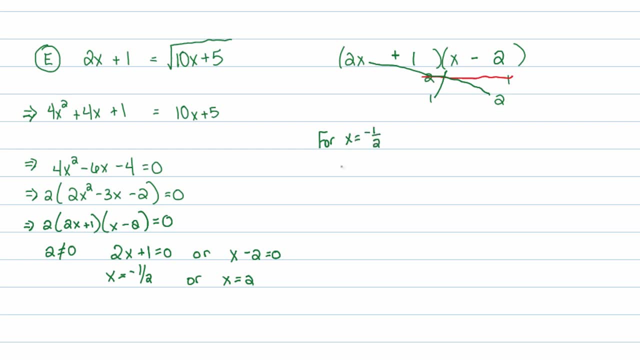 the x equals negative 1 half. when we plug that in, we have 2 times a negative 1 half plus 1, and that will be actually a negative 1 plus 1, or in other words 0 and the square root of 10 times a negative 1 half. oops. 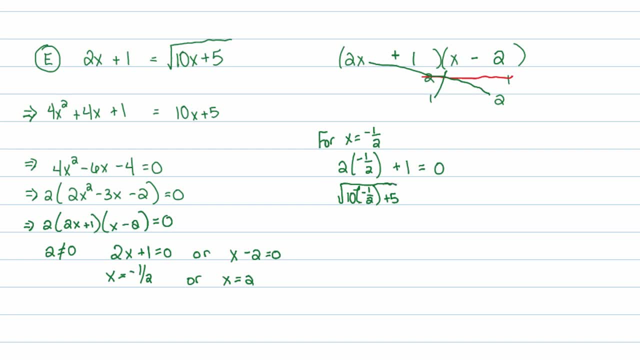 my handwriting's gotten sloppy. let's see: 10 times a negative 1 half is a negative 5, so that's the square root of negative 5 plus 5, which is actually 0. ok, so this does work out for this answer. and now let's. 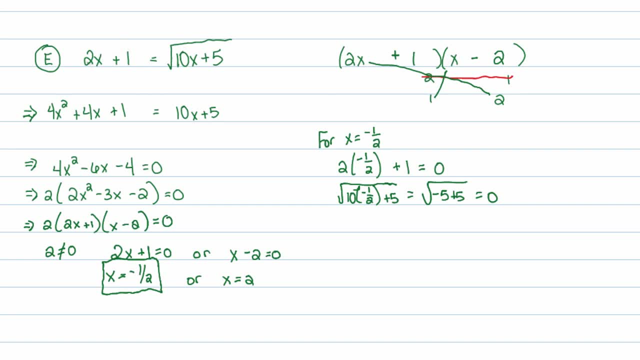 try the answer for. let's try: x equals 2. now you can do this mentally: two times two is 4 plus 1 is 5. ok, so left hand side will be 5. 10 times 2 is 20 plus 5 is 25. that gives. 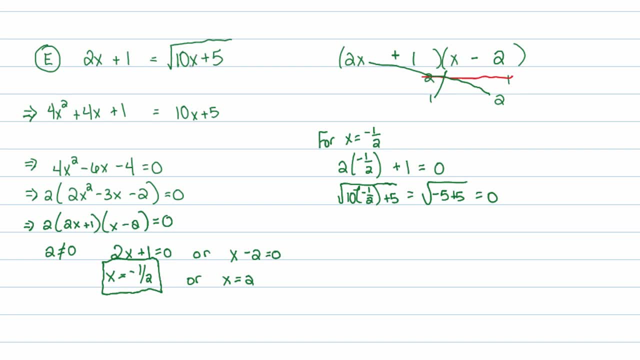 25 squared to 25 is 5, so we have 5 equals 5. that is also a grand old solution that works. so notice that we can have two solutions. that's absolutely fine. doesn't have to return an extraneous solution. and now you get to something like this: now we have two radicals right once you have two radicals. 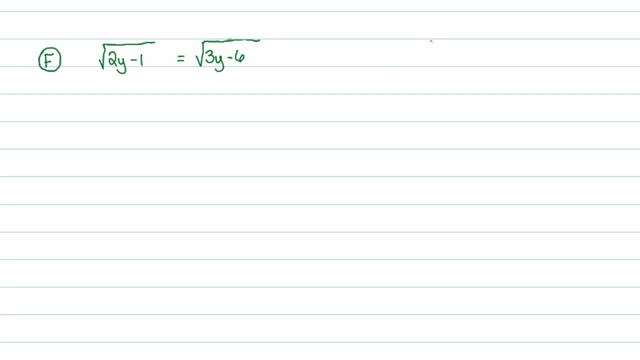 I know they can't combine. you can't remember that square root of a plus the square root of b- I'll see even say plus or minus square root of b- is not equal to square root of a plus or minus b. so you cannot combine radicals through addition or subtraction. just remember that. 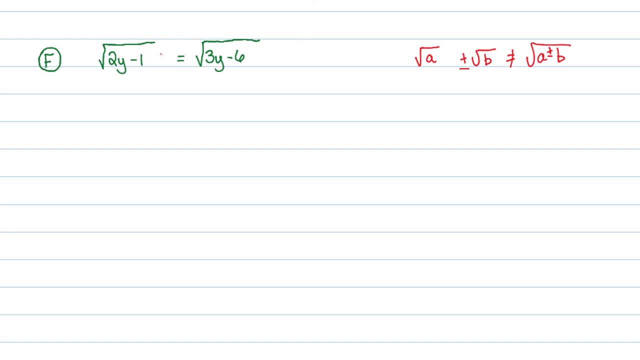 so these two will not be able to combine up. the best hope you have is to isolate one of them- which actually they're both isolated by themselves- on on their respective sides and then square both sides. so let me go ahead and square both sides. so if I square, I'll show the action of it. 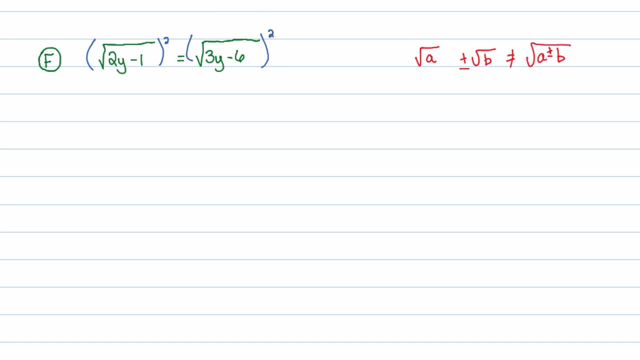 if I square the left hand side and then square the right hand side, I'll get: 2y minus 1 is equal to 3y minus 6. actually a pretty simple equation to solve right. subtract 2y from both sides, we get: y minus 6 is equal to a negative 1. 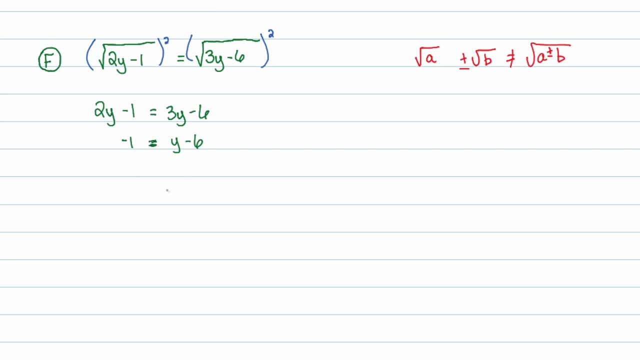 oops, my equal sign is a little messed up. and then add 6 to both sides, you'll get y. you'll get y minus 6 is equal to a negative 1 and y is equal to 5. now remember, we squared both sides of this equation. 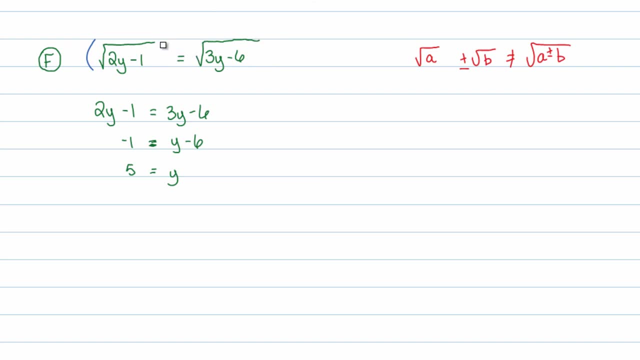 so we're going to have to check our answers. just clean this up so you can see where I'm checking my answer. I'm going to plug in 5 for y here, so that'll be the square root of 10 minus 1 or 9. 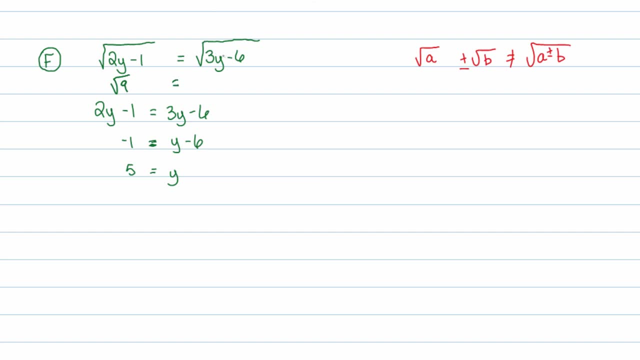 which we know is going to be 3, and plugging in 5, here we have 15 minus 6, which is also 9. so we root 9 equals root 9. that works out. there we go, so, even though I had two radicals in it. 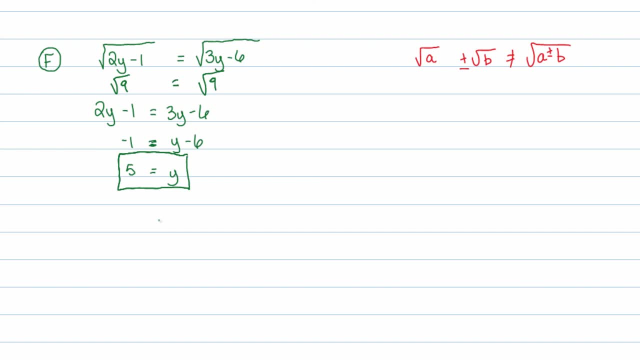 it's actually faster to solve, so let's try another one. okay, now we have something that's a little more challenging. we have: a radical is equal to a number minus a radical. I know things aren't going to combine, so I'm going to have two different terms involving variables here. 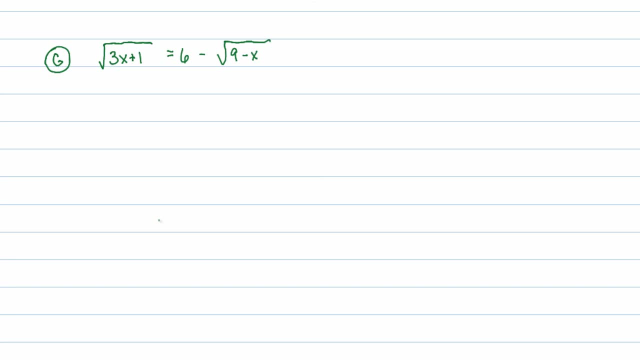 I have a term called the square root of 3x plus 1, and I have a term called the square root of 3x plus 1 and I have a term called the square root of 9 minus x, and neither of those cannot be combined up. 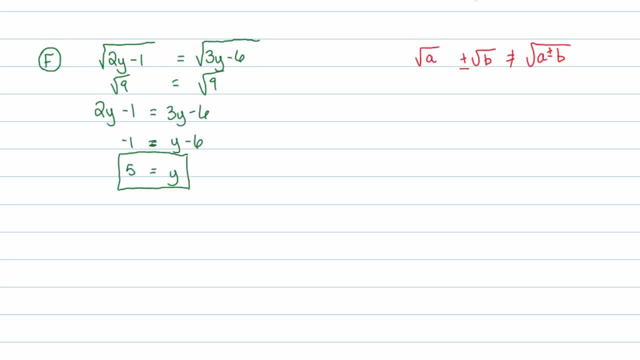 again because of what I just mentioned over here in red, that if I move them over to the same side you can't glue them together. remember, square roots can't be glued together through addition or subtraction. so this tells me I'm going to have to resort to special techniques. 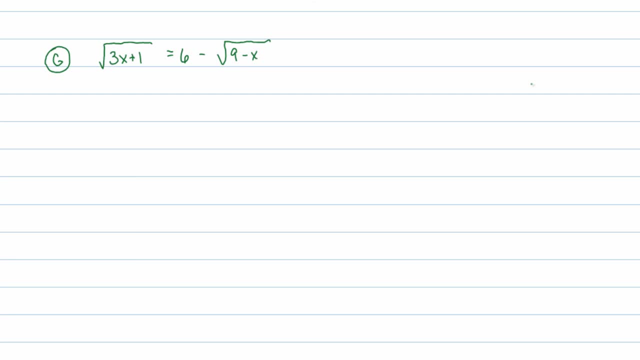 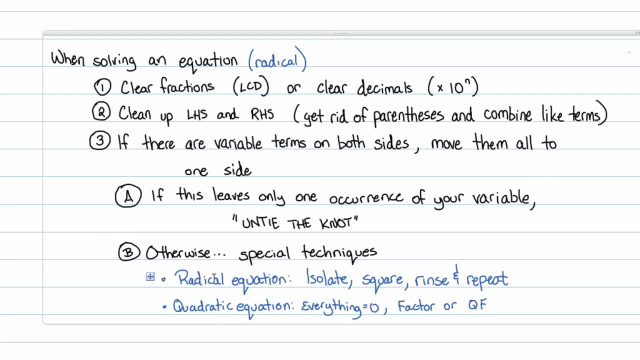 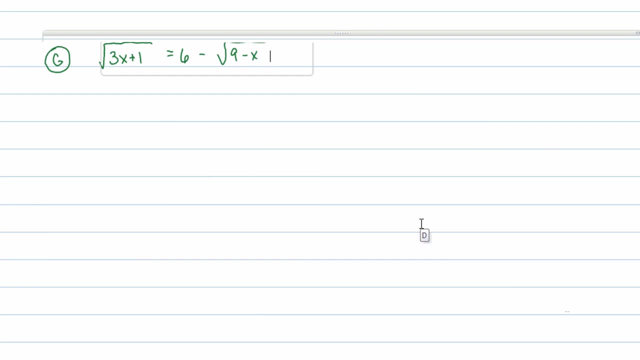 because I have more than one version of my variable. so special techniques for solving radical equations, as we've mentioned way back here, I'm going to have to resort to special techniques for solving radical equations, isolate one of them, square both sides, rinse and repeat if necessary. so I'm going to isolate one of them. 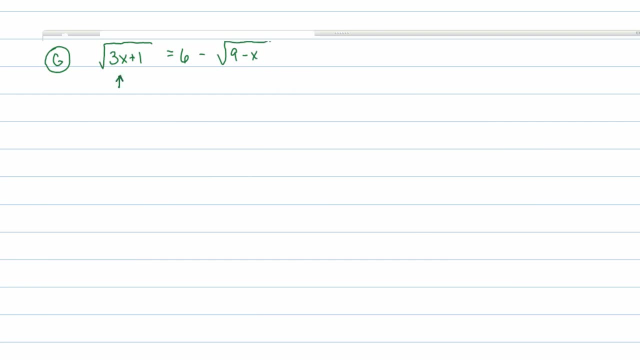 and one of them is already isolated. I will square both sides, so let me write that out slowly here. I will square the left hand side and I will square the entire right hand side. and again, be very careful when you do this. always remember what squaring means. 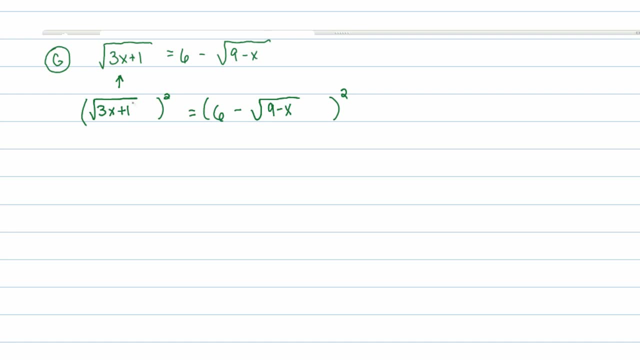 it means I have a picture and I'm multiplying it by itself. well, on the left hand side it just means you end up with 3x plus 1. let me write my implication signs in here. on the right hand side, it means I have 6 minus square root of 9 minus x. 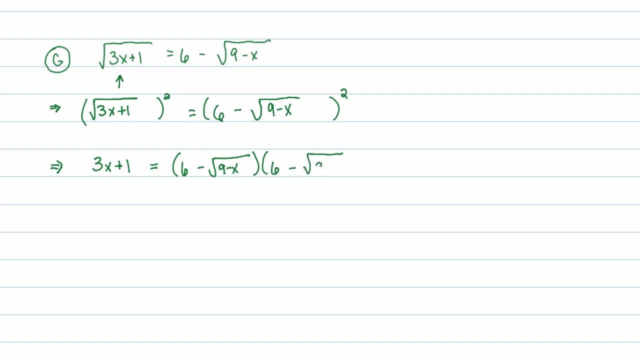 times the quantity 6 minus the square root of 9 minus x. in other words, it's this junk inside the parentheses times itself. so you're going to have to simplify this equation, simplify that right hand side. so let's multiply it out 6 times 6 is 36. 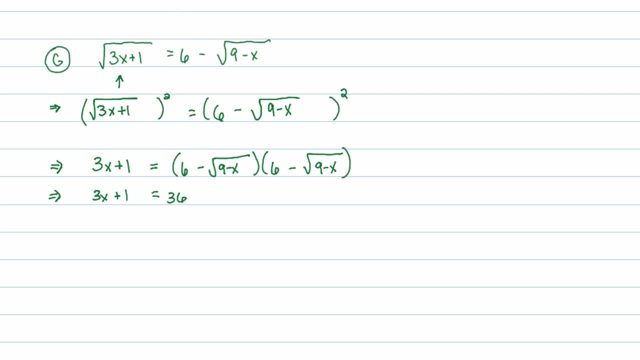 maybe I will even show you the color coding here: 6 times 6 will give me 36, 6 times a negative square root of 9 minus x is going to be a negative 6 times the square root of 9 minus x, 6,, I'm sorry, negative root. 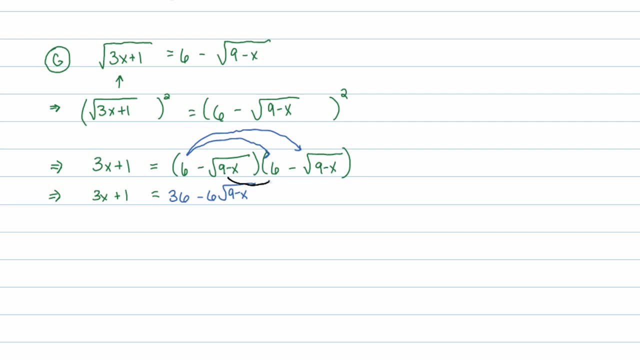 root 9 minus x times that 6 is going to be another negative 6. root 9 minus x. and finally, square root of 9 minus x times the square root of 9 minus x. they're both negative, so it becomes positive. and again: root 9 minus x. 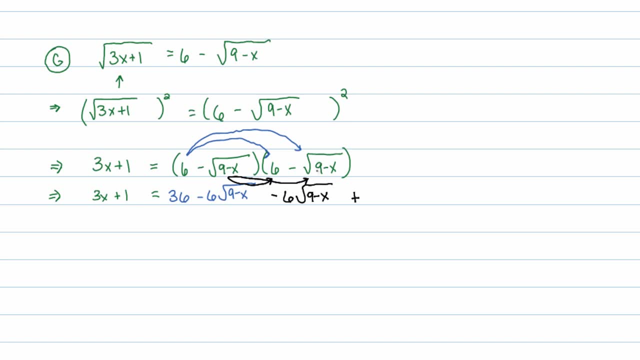 that's a half power of 9 minus x times a half power of 9 minus x, will have a full power of 9 minus x, or in other words just 9 minus x on the left hand, right hand side here. combine like terms. always simplify before doing a ton of calculations. 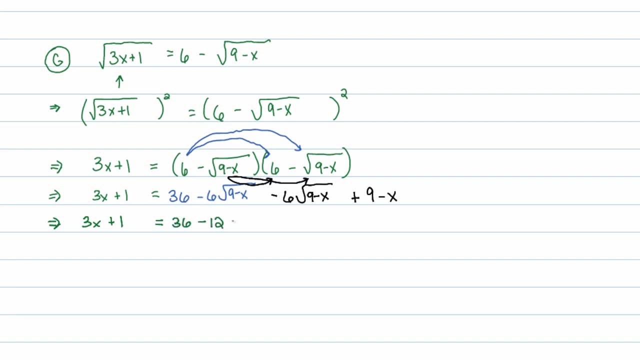 so it's going to be 36 minus 12. square root of 9 minus x: right, because I have a negative 6 of these pictures right here and I'm losing 6 more of the same pictures, so I've lost 12 altogether. and then finally, plus 9 minus x. 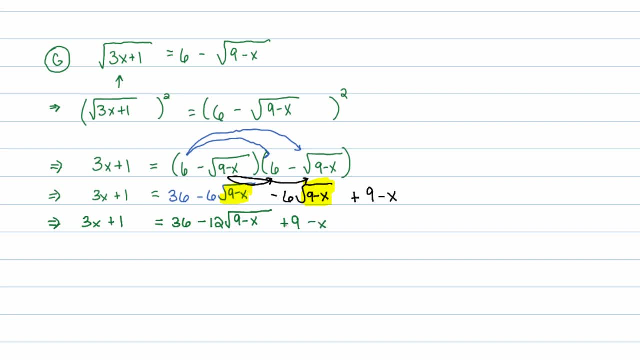 well, I haven't combined all like terms. actually. let me go ahead and add the 36. let me go ahead and add the 36. let me go ahead and add the 36 and the 9. here, 3x plus 1 is equal to 45 minus 12. root 9 minus x minus x. 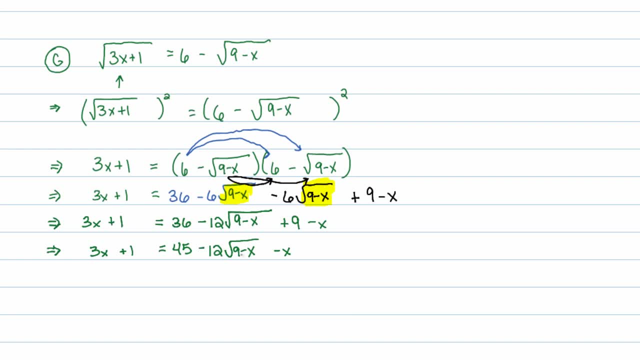 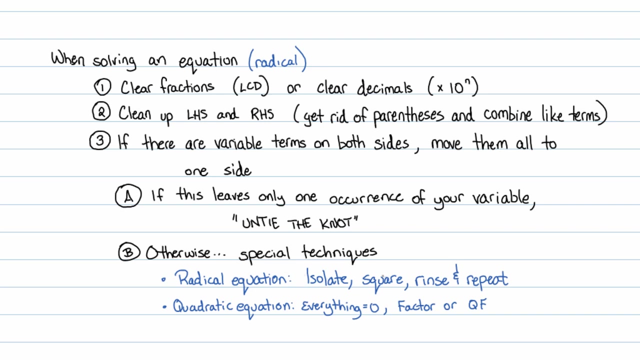 and I see I have a radical equation still because, see, I have a radical with a variable inside of it. so I'm going to isolate that radical, just like we've said way back, when we have a radical equation, isolate and we do a literal equation. here's a real advantage if you've done that. 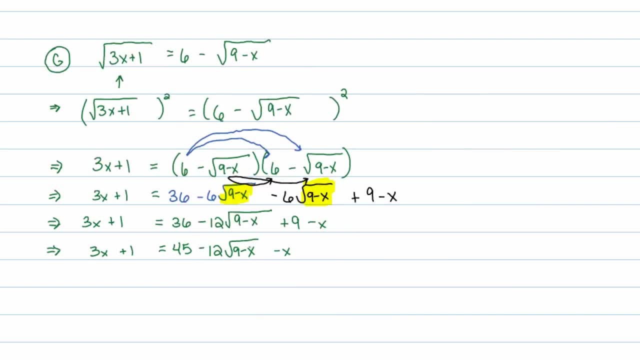 in the past, but this is just a little way to get better at this. you can see that the function of the equation is really simple. you don't have to worry that you have to know how to know how to solve this. the first step is to simply write the equation. 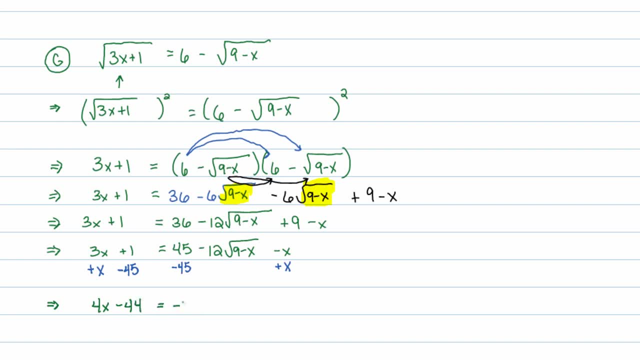 where the number of the roots are. you have to do the math, so you have to get the root of 4x minus 44 minus 4x minus 44, root of 9 minus x. There's arguments at this point. Some people might say to divide by that. 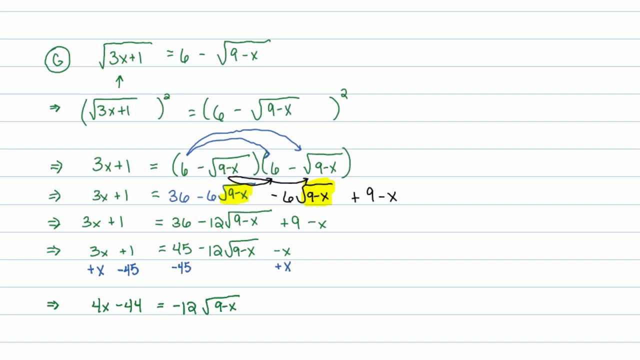 negative 12, and some people might say to not divide by negative 12.. I prefer to not divide by negative 12 at this point because you start getting fractions and I don't want to introduce fractions into my problem here. So instead I'm going to go ahead and maybe notice one more thing. 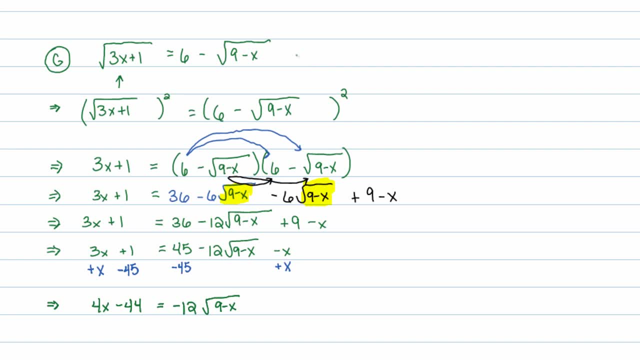 Now, what I'm going to do here is not critical that you do, but it does help out in your calculation a little bit. I'm going to notice that on the left hand side. well, first of all, I'm going to notice that all these coefficients- this 4,, this 44, and this 12- are all divisible by 4.. So maybe I'll just 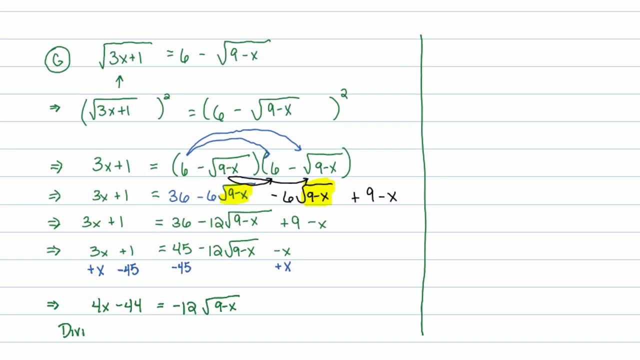 just to make the number smaller, I'm going to divide both sides by 4.. Sometimes making numbers smaller is such a good idea, So if you notice that, take advantage of it. So divide everything by 4.. So every term there by 4 you'll get. x minus 11 is equal to a negative 3 times the square. 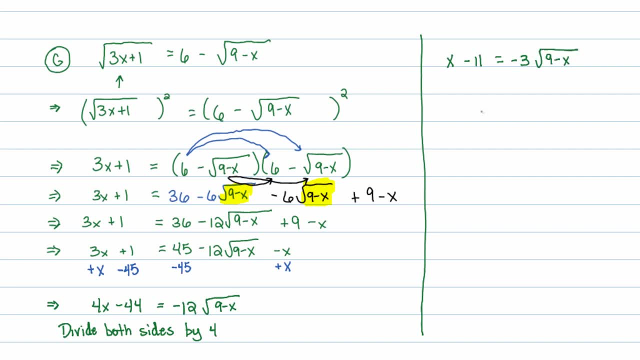 root of 9 minus x. And now I will square both sides. And again, I'm not going to divide by a negative 3, even though some people swear that you should, or something like that. The fact is, if I divide by a negative 3, I'm going to get fractions and I don't want to deal. 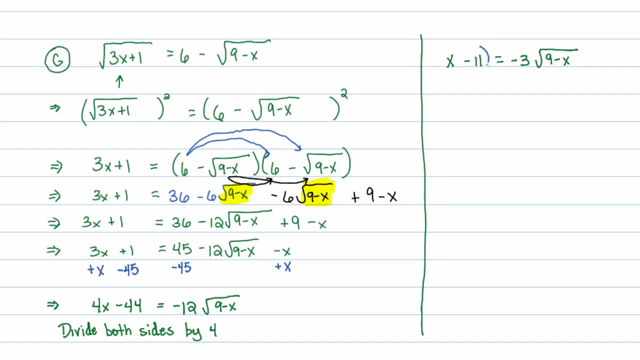 with fractions, So I'll just square both sides: Square the left hand side, square the right hand side. Now, the only thing you have to remember is that you have two different kinds of squaring actions going on here You have one. you're squaring a binomial, So that's x minus 11. 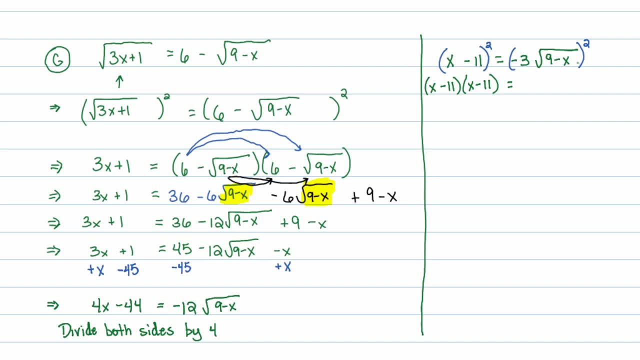 times x minus 11.. And on the right hand side you're squaring the product of two numbers, So you have that negative 3 being squared times the square root of 9 minus x being squared. Now the left hand side distributes out to x squared minus 20 times the square root of. 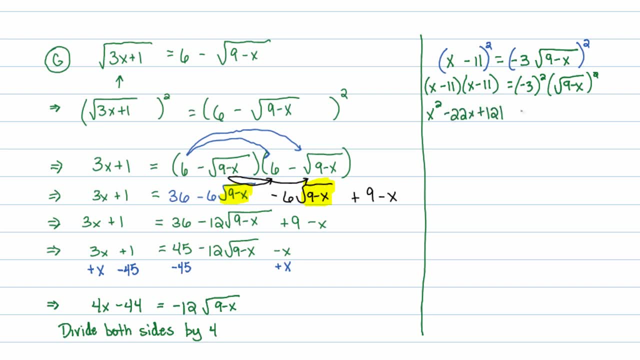 22x plus 121 equals- the right hand side is 9 times the quantity, 9 minus x, because the square and the square root cancel each other out. Let me distribute that 9 through A lot of little paperwork here: 81 minus 9x. I see this is quadratic in the end, so I'm going. 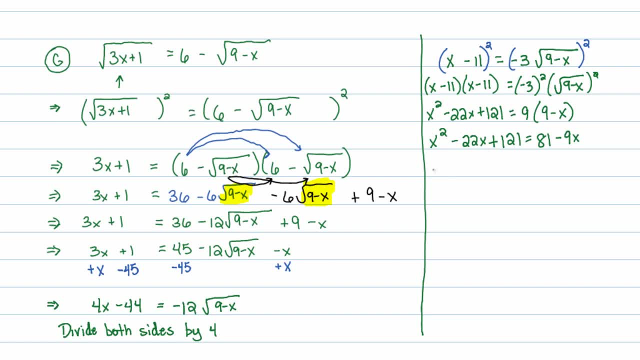 to go ahead and isolate everything on one side. So I'll have x squared minus 9x, And I have x squared. Let me see I'm going to add 9x to both sides, So negative 22 and adding back 9 would give me a negative 13x. Let's see, Just double checking my work And then: 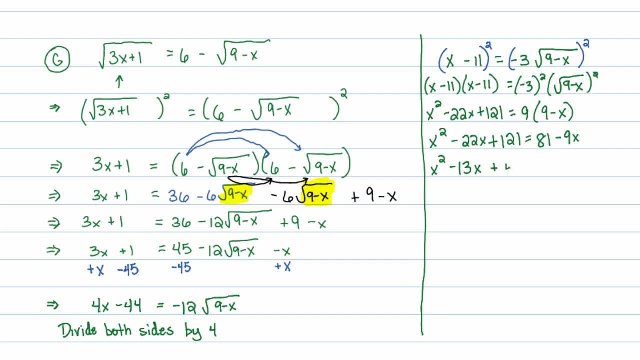 subtracting 81 from both sides means that I'll have a positive 40.. Now, this is the easier kind of factoring, because you're just looking for two numbers that multiply to 40 and add to a negative 40.. Although divided by eight, developed the. 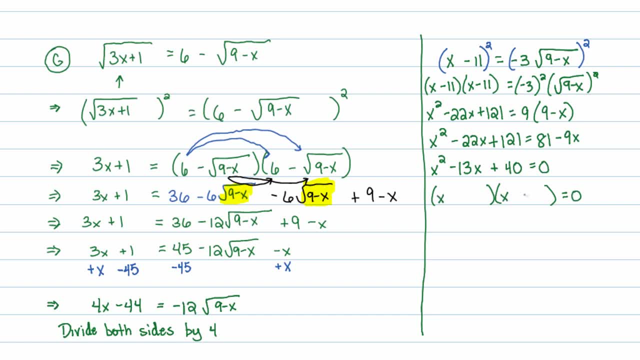 negative 13.. Well, that would be negative 8 and a negative 5, maybe. So we have two options for x. Either x is equal to 5 or x is equal to 8.. Both could be true. one could be true or none could be true. The way you find out which one is true, or if any of those is true: 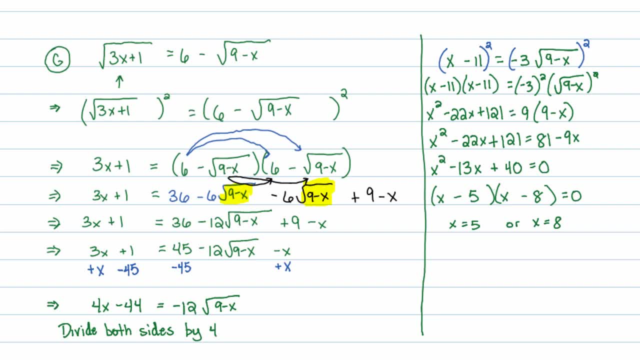 is you plug those back into the original equation here. Make some room. So if I plug in the 5, I'll get 15 plus 1 or 16.. So on the left hand side I have the square root of 16, which is 4.. 6 minus. On the right hand side I have 6 minus and then the square root. 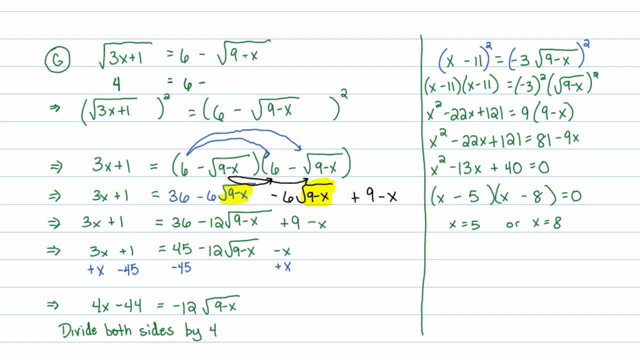 of 9 minus 5.. 9 minus 5 is 4, square root of 4 is 2 and if you look at that, that is true. Just checking really quickly, that works out. This is why you have a rewind button by the. 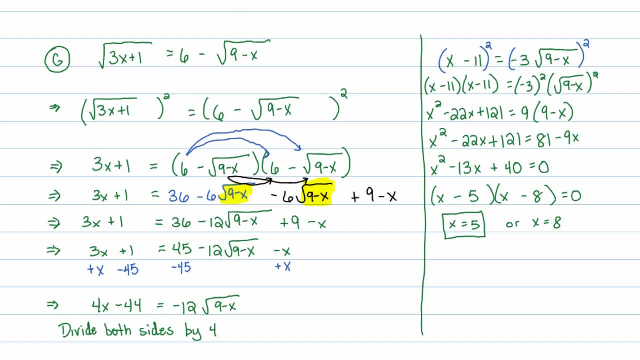 way, So that you can kind of pause it, go back and figure out what I talked about. I talked kind of quickly, So let's plug in: x equal to 8.. 8 times 3 plus 1 is a 25.. Square root of 25 is 5.. I want. 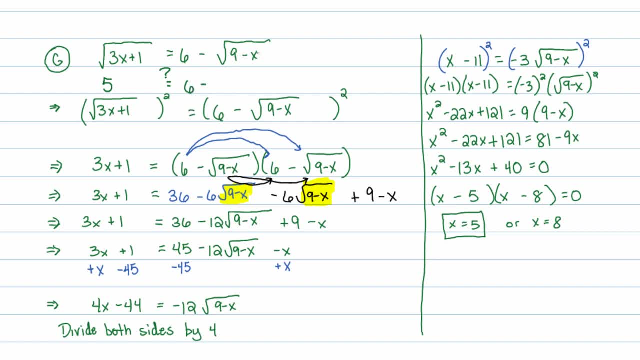 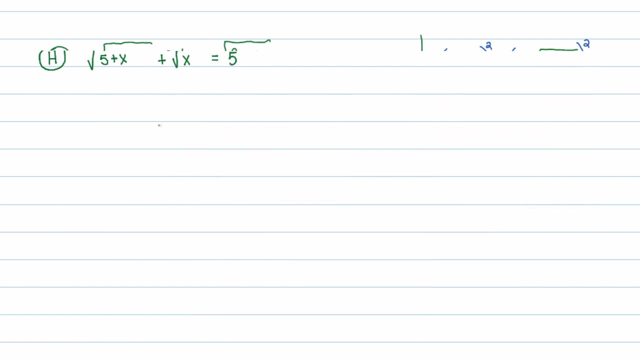 to know if this equals 6 minus the square root of 9 minus 8.. Square root of 1, which is 1.. five equal to six minus one? yes, it sure is. so here is another solution, not extraneous, as a final example for solving radical equations. this is kind of like the ultimate style of 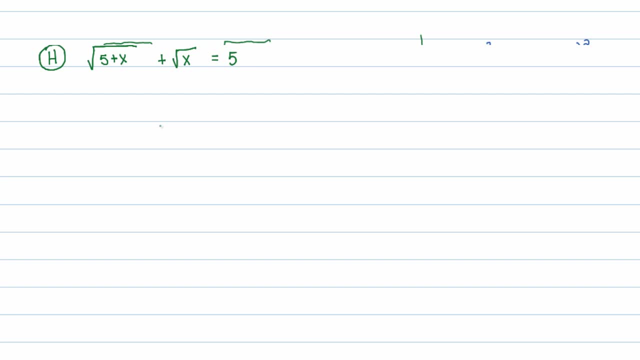 equation, even though it looks somewhat harmless. the only reason why i consider this to be a more difficult equation is just because, well, two radicals are on one side. they can't combine, and so you know you're going to have to resort to special techniques, and the special 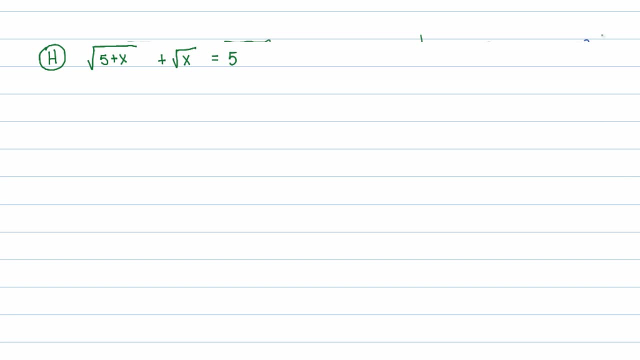 techniques. remember. say that if you have a radical equation, you have to isolate one of the radicals first. that's probably the biggest mistake i see, as students don't isolate a radical. so you could isolate either of these radicals. i'm going to show you the right one. 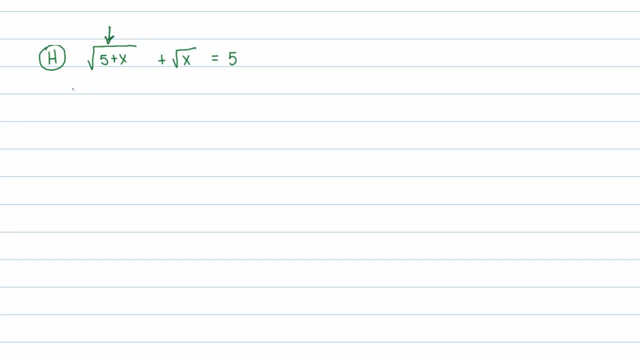 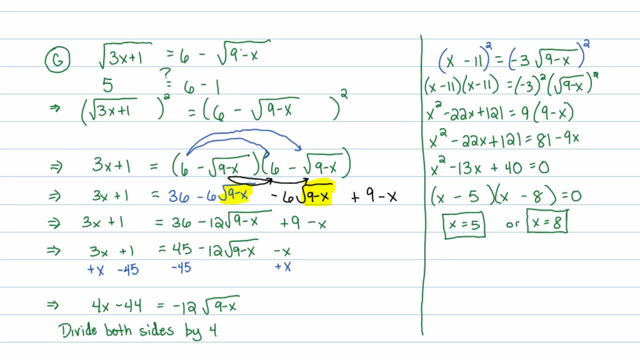 to isolate. i would isolate this guy right here. the only reason why is if you look here, is if you look in the top right of your dictionary and you have some radicals that are on either. look back at our previous example here if notice that when we squared both sides, we had the square. 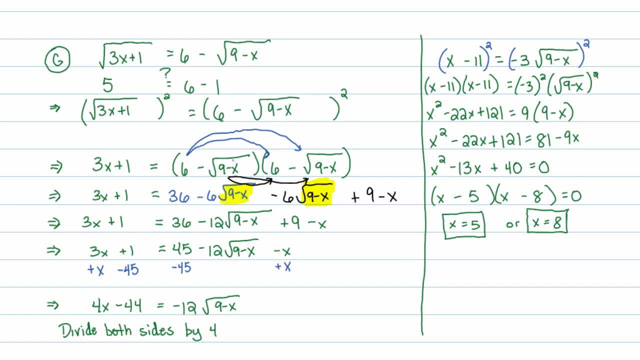 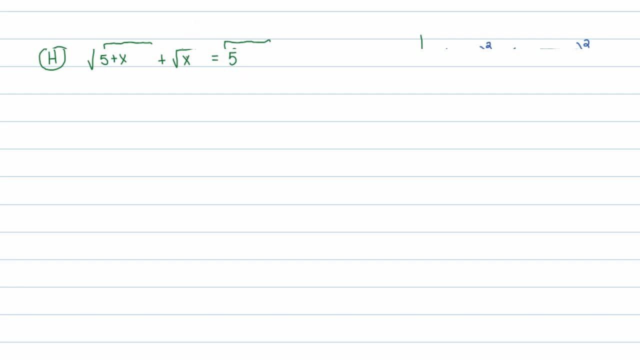 root of 9 minus x inside the squaring and it just created this mess, okay. well, if you have the choice of having to square something in the long run, well, maybe i should just show you. let's subtract root x from both sides, so here's root 5 plus x is equal to 5 minus the square root of x. 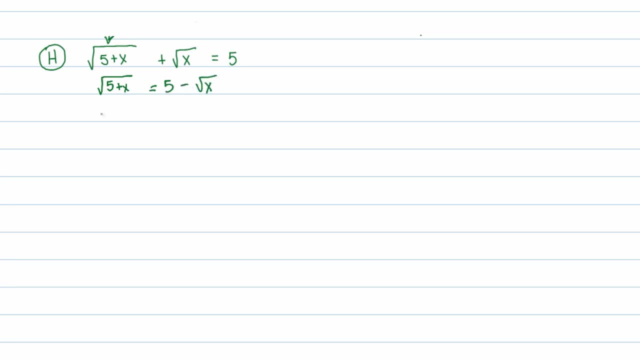 and now i'm going to square both sides. so if i square both sides, i'll show the action right here. squaring and squaring, i get 5 plus x on the left hand side. on the right hand side i get 25 minus 10, root x plus x. and now what i'll do is i'll subtract x from both sides. 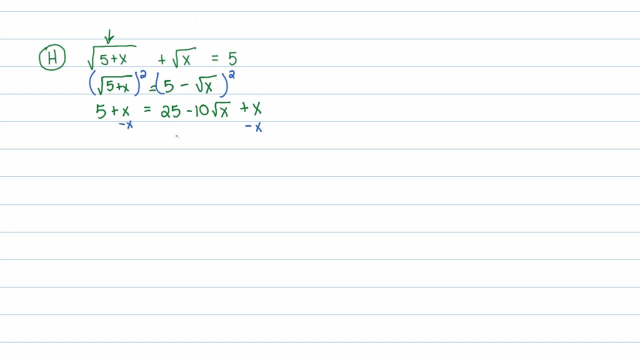 and i'll subtract 25 from both sides and i get, let's see, on the left hand side, the x's cancel. and also, 5 minus 25 is a negative. 20 equals 25 minus 25, that's gone. and x minus x, that's gone. and actually, since 10 does go into 20, nicely, i'm going to divide. 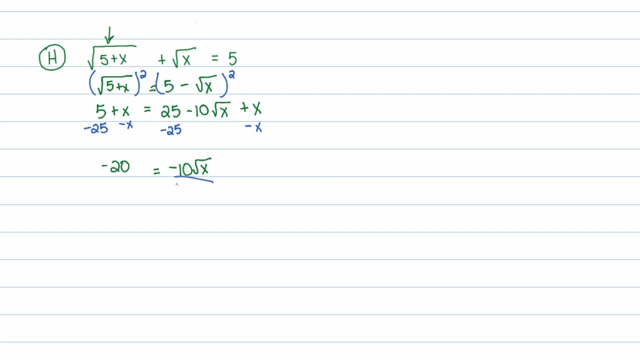 both sides by a negative 10. here let's divide this side by a negative 10, this side by a negative 10, and i'm going to divide both sides by a negative 10 and i'm going to divide this side by a negative 10. 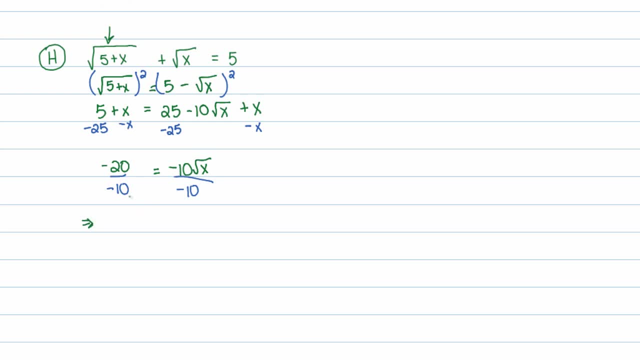 you will see that we get. what is it? square root of x is equal to 2.. So that means that x is equal to 4 when you square both sides. So if you check that out and see if that's true, it actually is right. 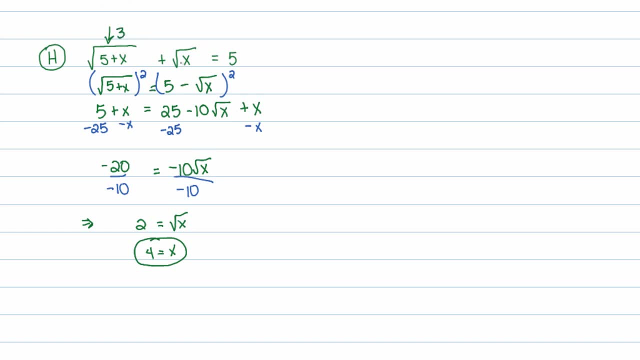 5 plus 4 is 9, square root of 9 is 3, plus square root of 4 is 2, 3 plus 2 is 5.. Okay, great, that does work out. Now let's suppose that you had done this problem the other way. 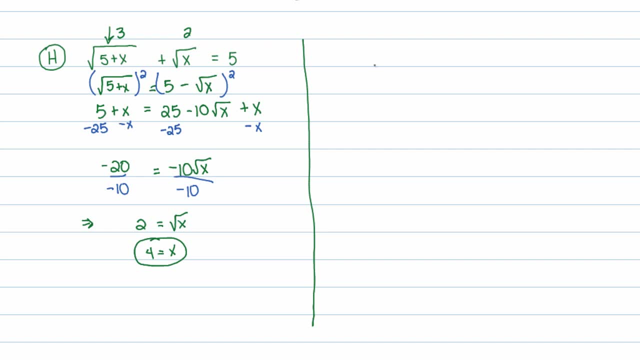 where you said: oh, you know what I'm going to do. instead, I'm going to isolate the square root of x, because that looks like such a better isolation. It's not. It's a little uglier actually. So let's see what happens and why I consider it an uglier isolation. 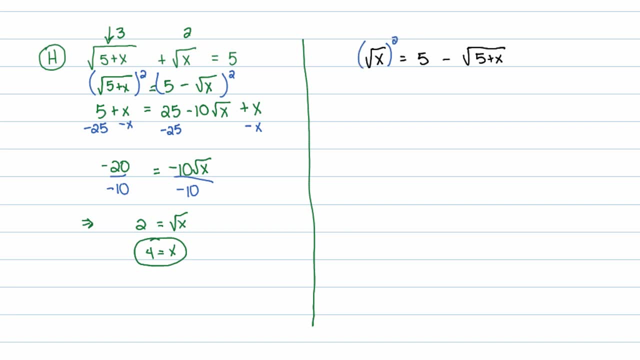 I'll first square both sides, which is the same in both cases. actually, All the steps are the same. it just looks uglier in the end. Square Squaring the square root just gives me x. When I distribute this out, I'll get 25 minus 10 root, 5 plus x plus 5 plus x. 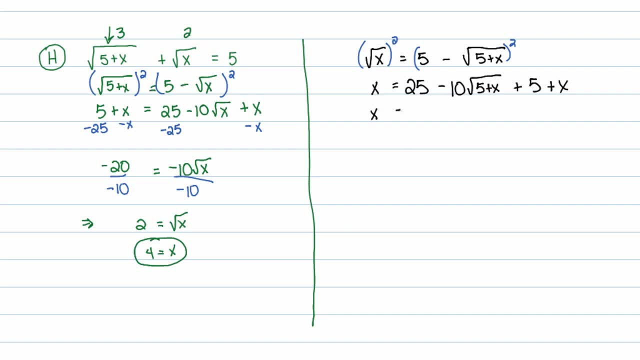 Let's combine like terms on the right-hand side, So I'll have 30 minus 10, root 5 plus x and then plus x. Let's subtract 5 from both sides or x from both sides, I'm sorry, And. 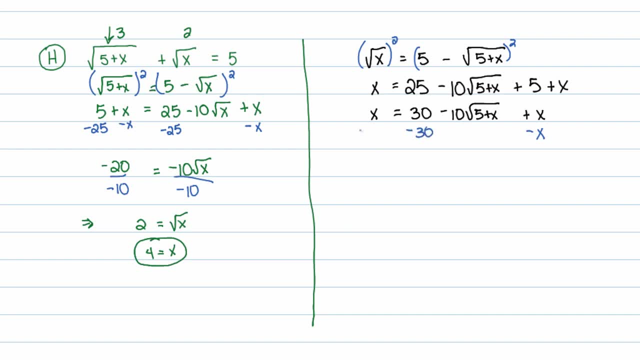 And a 30 from both sides, So subtracting x and a 30. There was just a 0, no numbers over there, so no numbers minus 30. It gives me a negative 30.. Equals, What is this? 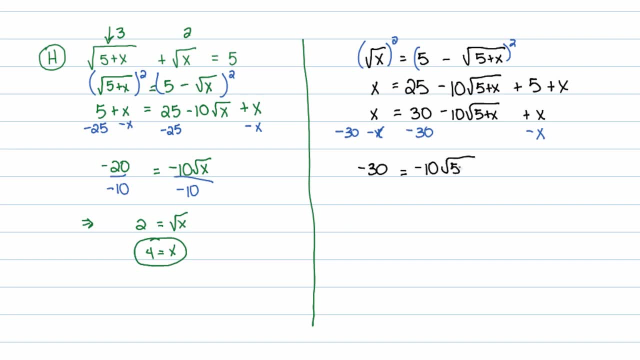 A negative 10 square root of 5 plus x. Divide both sides by a negative 10.. You'll get 3 is equal to root 5 plus x. Square both sides, you'll get 9 is equal to 5.. 5 plus x. 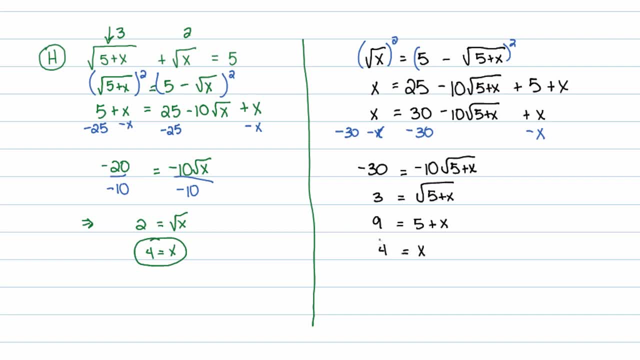 Subtract 5 from both sides you get: x is equal to 4.. Check your work Now notice we get the same answer. But there were quite a few more steps actually This one. we had the isolation step, Then we had the squaring step. 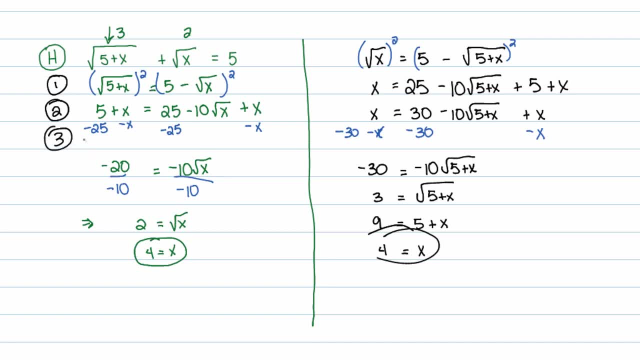 We had the combining like terms, or basically moving everything to the left-hand side step, And then we divided and squared Together To get the answer Here. I moved everything over, I multiplied out, squared both sides. I had to combine like terms actually first. 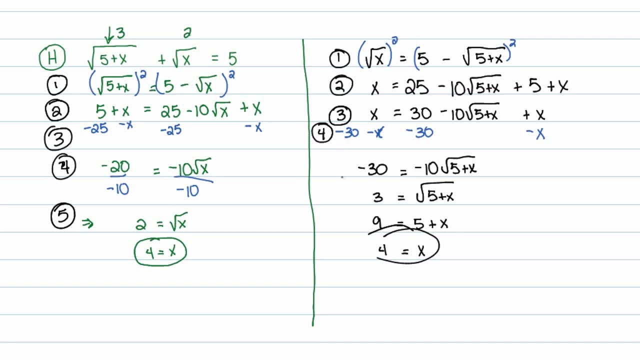 And then I was able to do all the subtractions, And then I did this little division here, And then, once I did the division, let's see These two steps are combined. So once I did the division, I still had to do a squaring step. 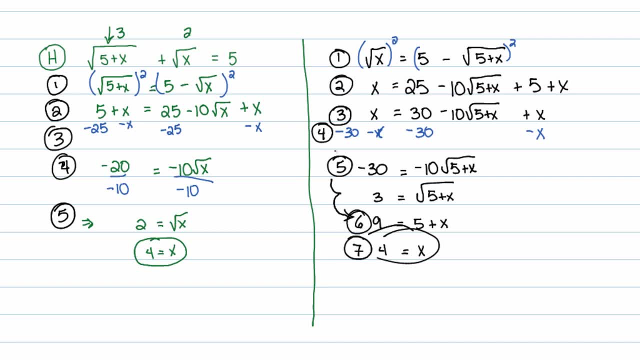 And then do another like subtract 5 from both sides. So there's 7 steps doing it this way. So rule of thumb is: if you have a radical equation, it's a good idea to the first one to isolate, for is the one that has the most difficult stuff in it. 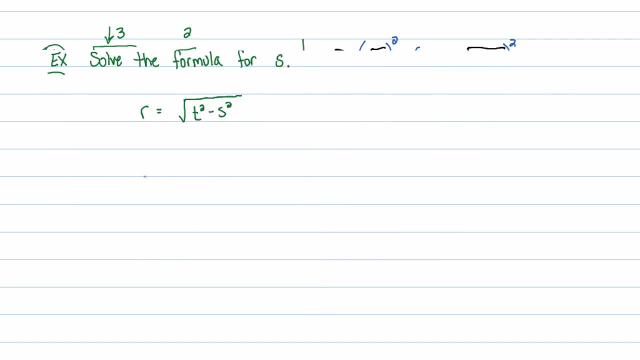 Okay, That's a good rule of thumb. Now I'd be remiss if I didn't do a formula solving problem, So let's solve this formula for s Now. notice that s only occurs once in this entire equation. It's right here. 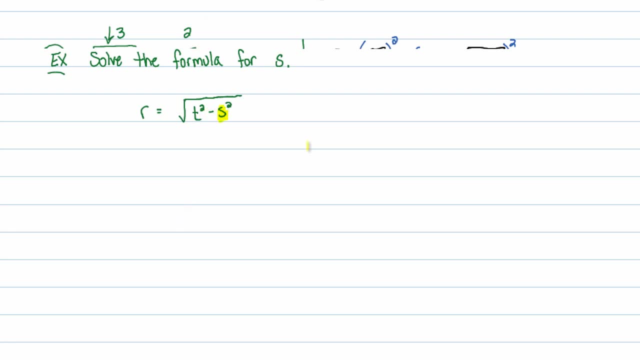 It's being squared, but whatever. So if you're asked to solve for a variable that only occurs once, you could just list out what happened to s And then, once you list it out, you can undo it. So first thing that happened to s is it got squared. 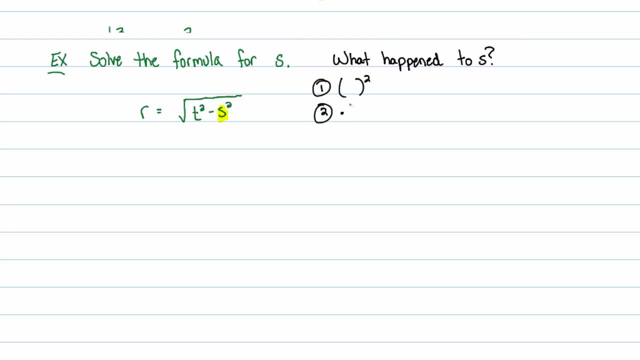 The second thing that happened to s is it got multiplied by a negative 1, actually because there's a negative attached to it. And then the third thing that happened after we attached the negative to it was we added t squared to it. 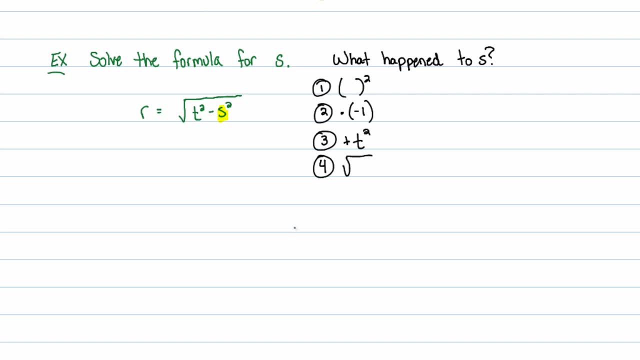 Then we took the square root. So notice all those things that happened to s. So we're going to have to solve for s by undoing these things. So the first thing I'm going to do is undo the last thing they did. 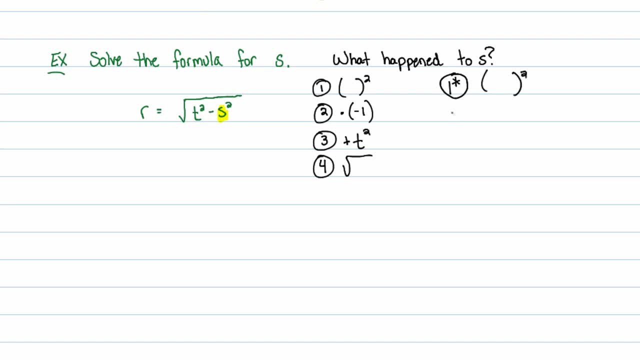 I'm going to square both sides, because they took the square root of both sides And then they added t squared. I'm going to subtract t squared. Then they multiplied by a negative 1.. I'm going to divide by a negative 1,, although multiplying and dividing by a negative 1,. 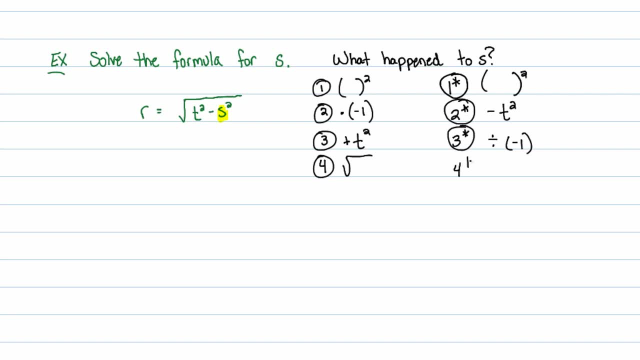 are the same thing, And then, finally, I will have to take the square root of both sides. So let's go ahead and do these right here. So the first thing I'm going to do is square both sides. Now, when you're dealing with formulas and a bunch of variables, 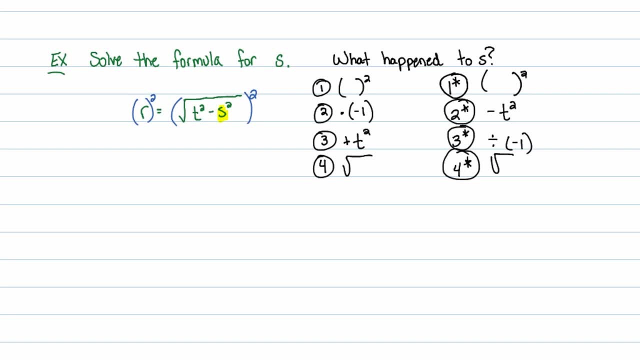 you're not really going to mention the fact that you possibly have an extraneous solution. It's just not going to happen here, So you don't have to worry about that. So we just get: r squared is equal to t squared minus s squared. 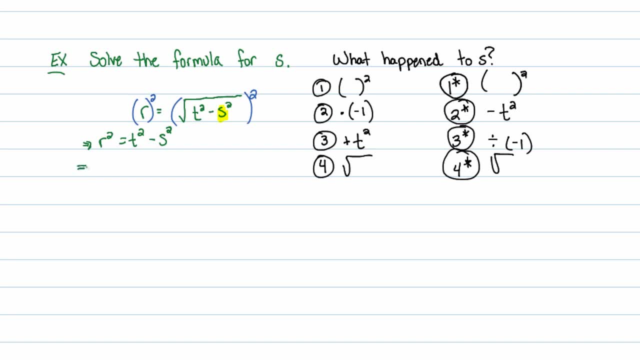 I tell myself: now I'm going to subtract t squared from both sides, because we've just finished this step. So r squared minus t squared is equal to a negative s squared. Then I tell myself that I'm going to divide both sides by a negative 1,. 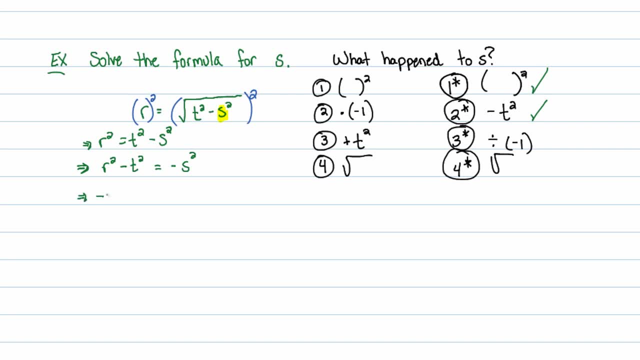 which essentially means just flip the signs on everything. So I have a negative r squared plus t squared is equal to positive 1. So I'm going to take the square root of both sides And the square root. remember, if you're solving for a variable s and it's being squared. 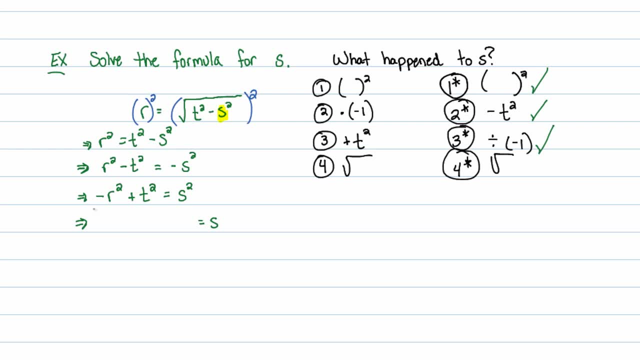 when you take the square root of both sides, remember the other side is going to be plus or minus the square root of negative r squared plus t squared. That's as good as it gets. You can't really do anything else with that. 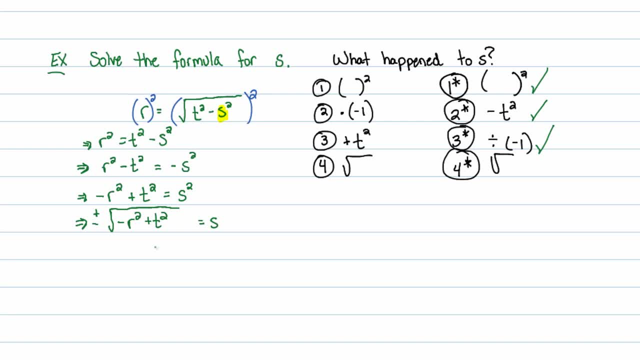 By the way, this video took me three days to record. I've been, I've had pneumonia, So, but I made it through it.